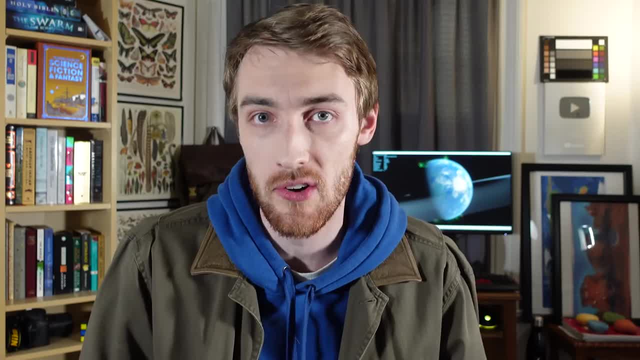 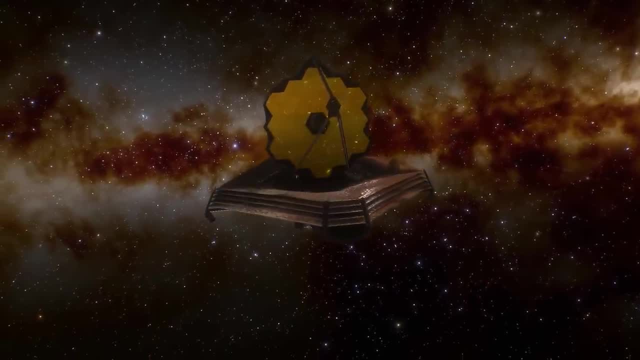 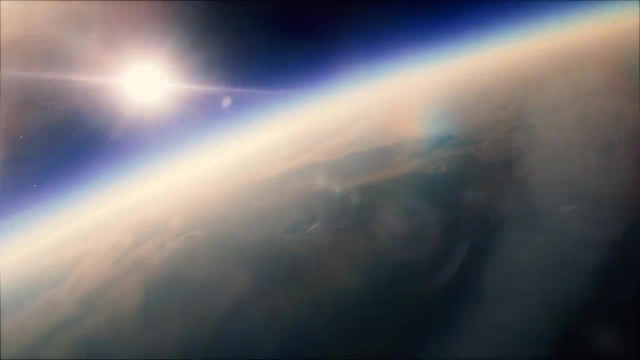 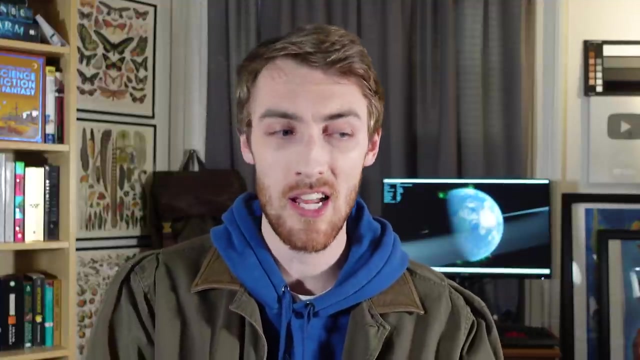 not to find habitable exoplanets, but rather simply to familiarize ourselves with those closest to us so we can figure out which ones we should be paying more attention to and see if we can come to any conclusions about our cosmic neighborhood. Okay, before we get started, I just want to make two things clear. First, everything. 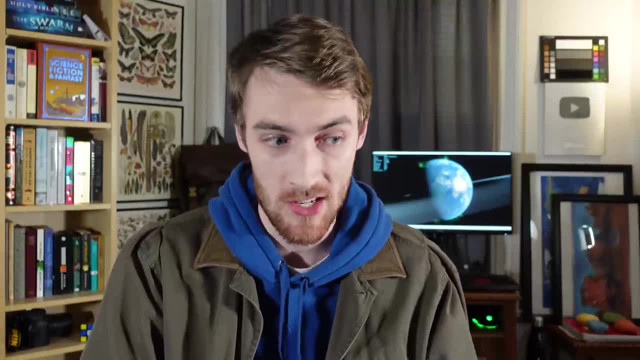 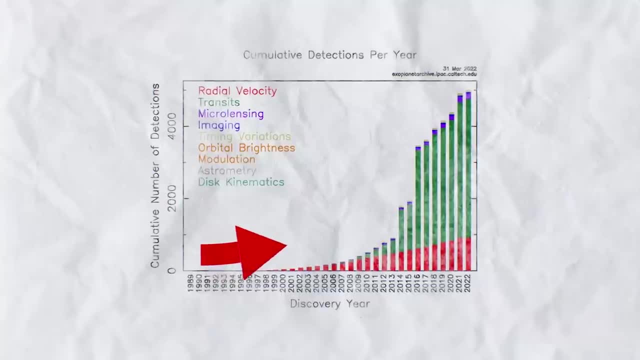 I talk about in this video is subject to change and likely will change as we continue to gather information and make more educated inferences. Right now, we live in an age of rapid discovery and advancement. If not, let me know how you privacy is. We might join up and face the best by doing. 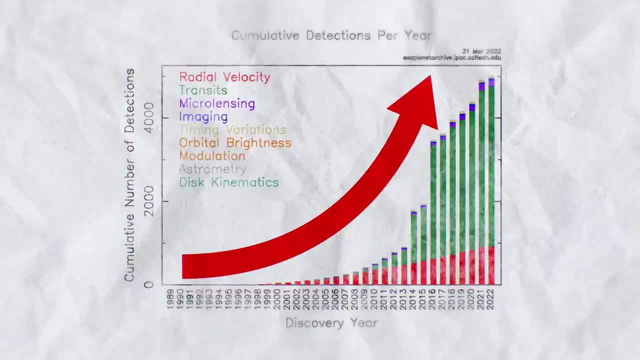 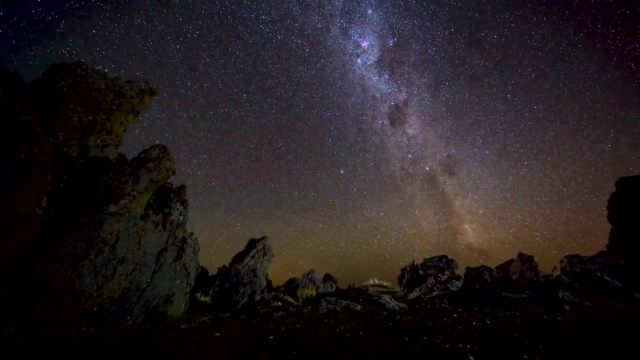 And because of that, I'm sure in almost no time at all this video will become drastically outdated, both because of what I say about individual planets, but also for all the really interesting ones that I'll likely skip over because they're yet to be discovered. 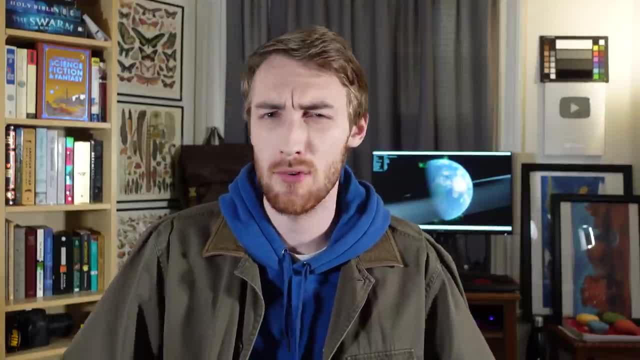 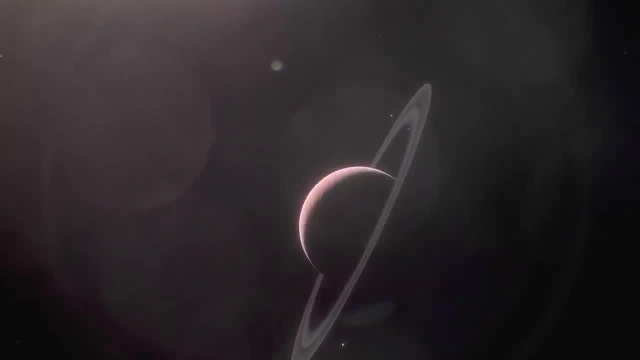 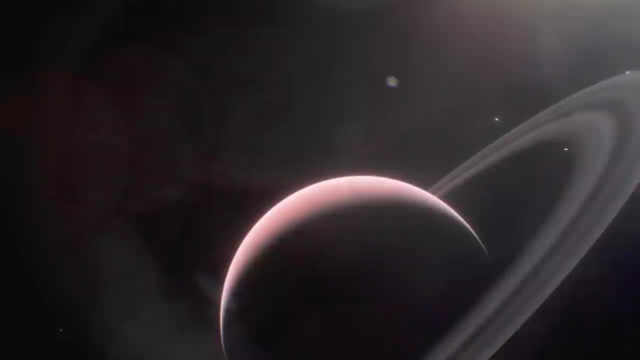 And so the selection of planets we look at today should be considered more of a random sample than an all-inclusive list. And two, if it wasn't already clear at this point, we know very little about all of these places, and so any depiction of them can't be considered anything more than an artistic interpretation. 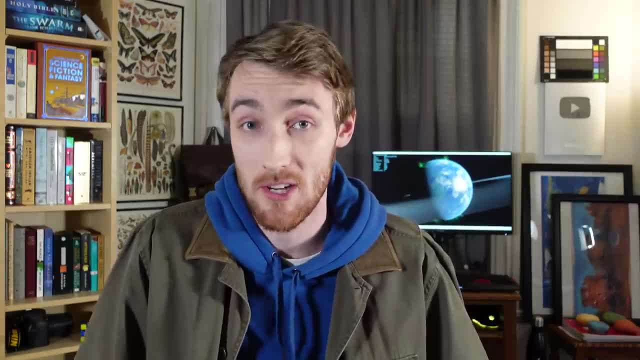 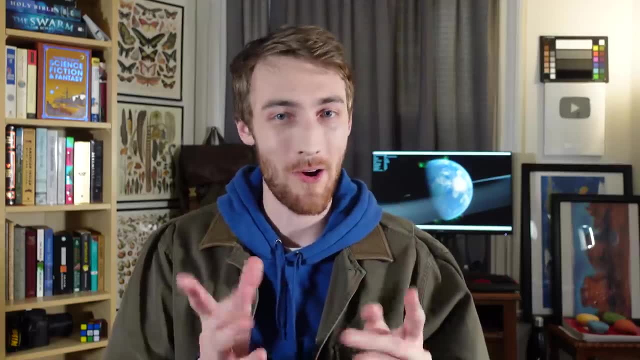 I mean, I think I did a reasonably good job at using the information at hand to portray these planets, but of course I also had to fill in a few gaps, so just keep that in mind. Got it Okay, cool, Then let's get started. 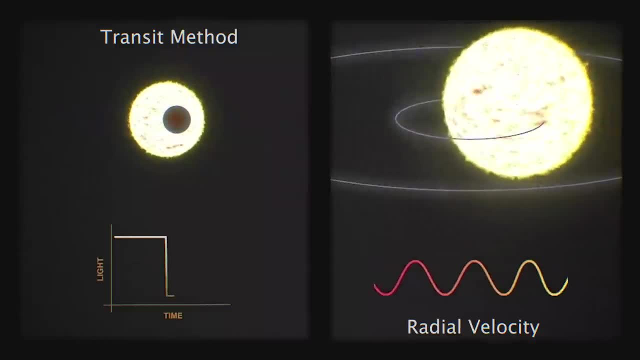 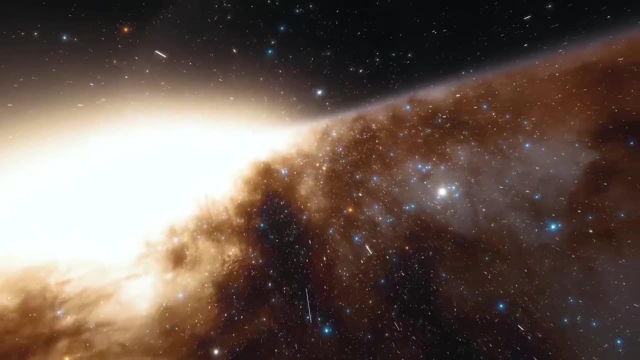 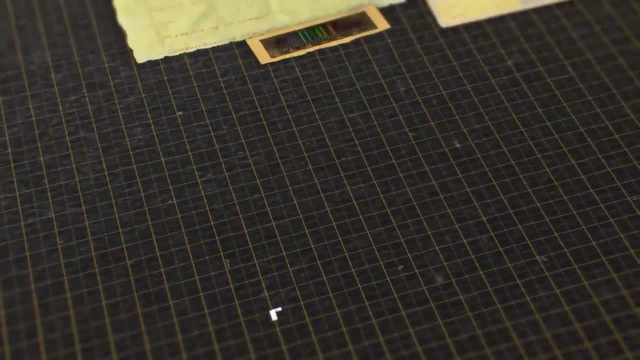 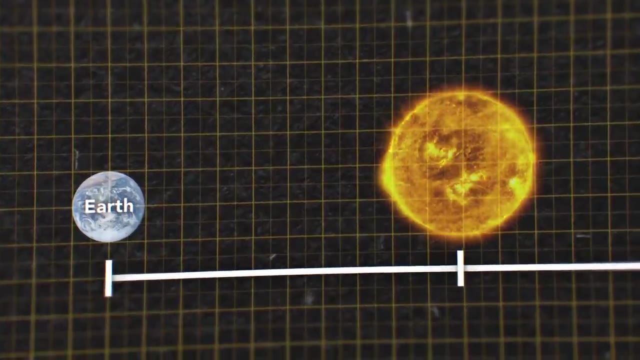 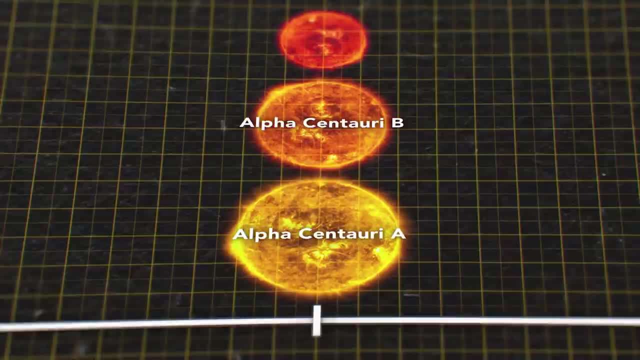 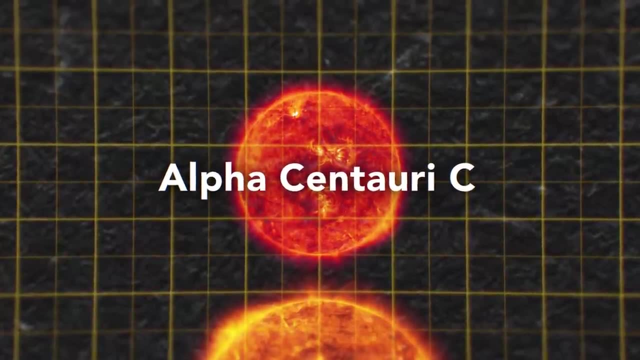 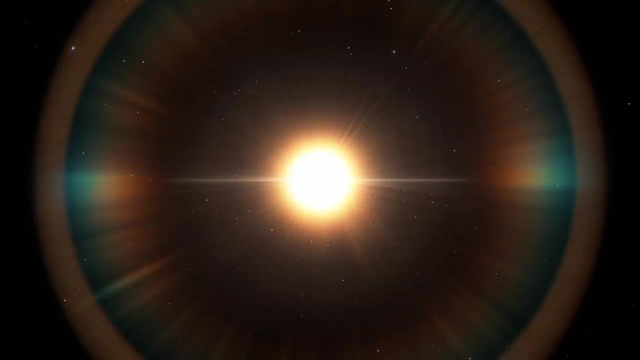 light forms the third brightest star in our sky, while the third, Alpha Centauri C, is a much smaller and dimmer red dwarf that can't even be seen from Earth. But Alpha Centauri C has another name, Proxima Centauri, alluding to the fact that this is the closest star in our proximity. 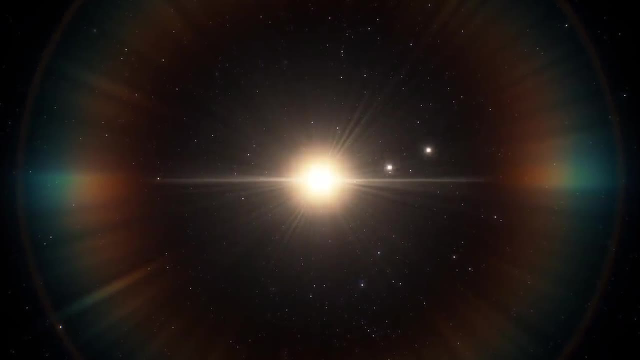 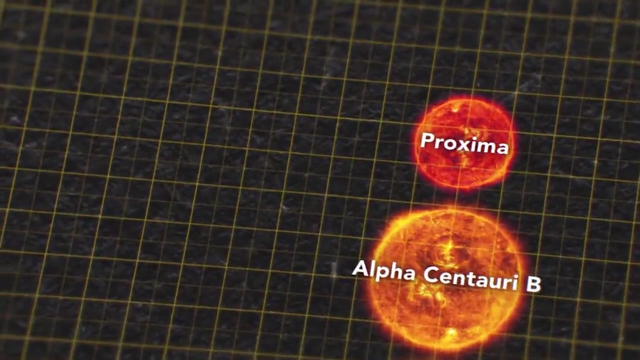 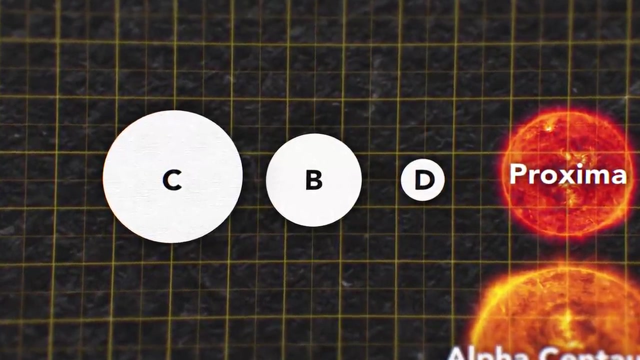 And it's here, around this faint ball of burning gas, that we'll find the Alpha Centauri C. Remarkably, a total of three planets have been found in orbit around Proxima Centauri, aptly named Proxima B, C and D, and perhaps even luckier than that, one of them, Proxima B, sits within its star's. 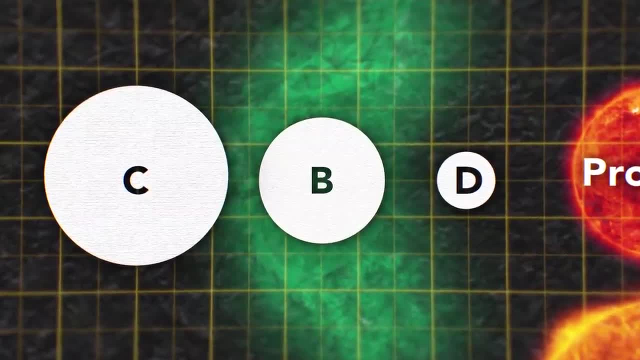 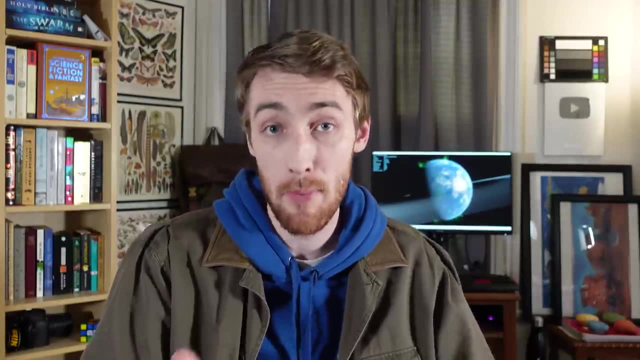 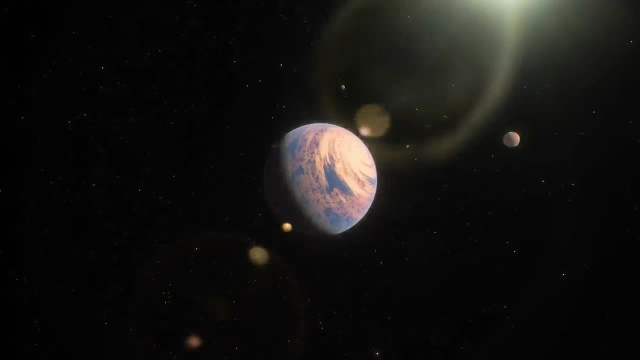 habitable zone where liquid water is theoretically possible. Now, technically, I already talked about Proxima B in the first exoplanets video I made, but I'd like to appreciate how miraculous it is that the very closest star to us just so happens to also host a potentially habitable world. 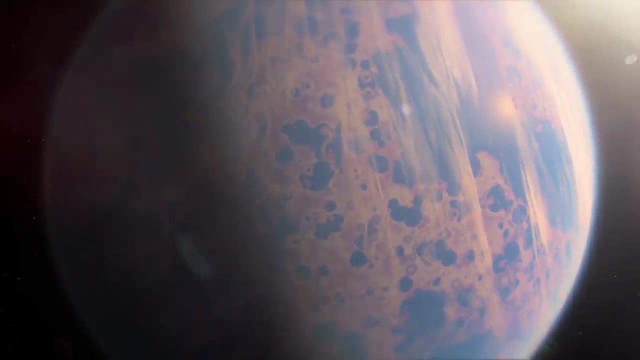 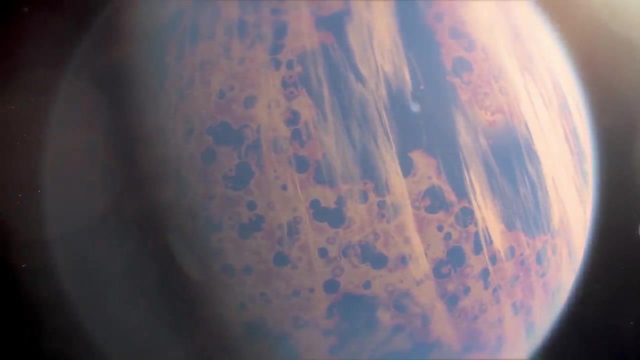 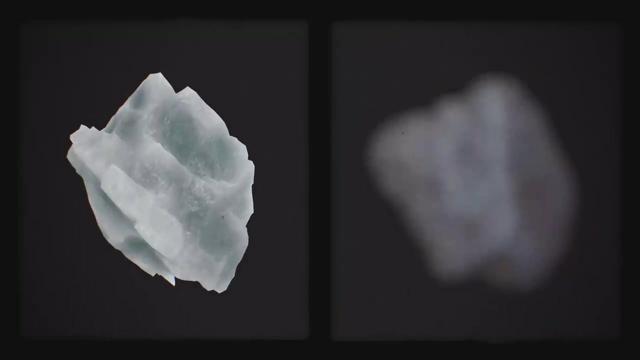 With a mass almost identical to the Earth's. this suggests Proxima B is a rocky planet, while its relatively larger estimated radius appears to suggest its density is far lower than the Earth's, meaning the planet's composition likely features more lightweight compounds like water rather than heavier elements like iron, indicating this may in fact be an oceanic. 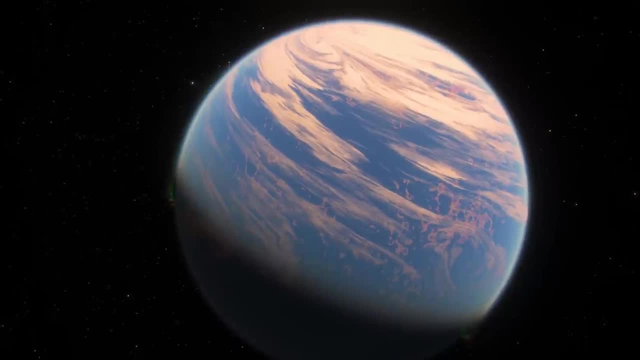 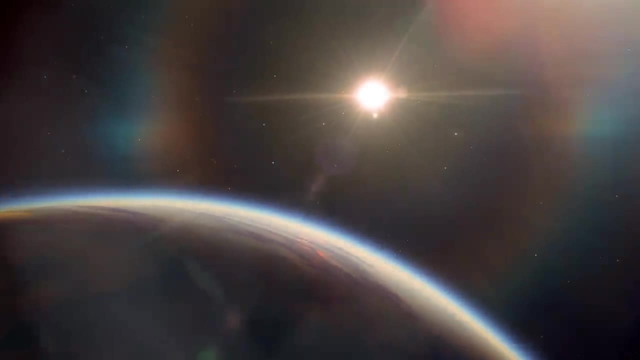 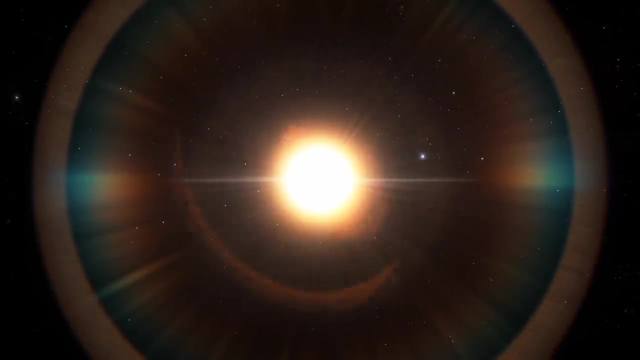 world and only helps to improve its chances of harboring life. However, surviving around Proxima Centauri wouldn't exactly be easy, thanks to its nature as a flare star, every so often releasing huge bursts of radiation many times greater than its typical output, bombarding any and all nearby planets with enough energy to strip even a thick atmosphere and 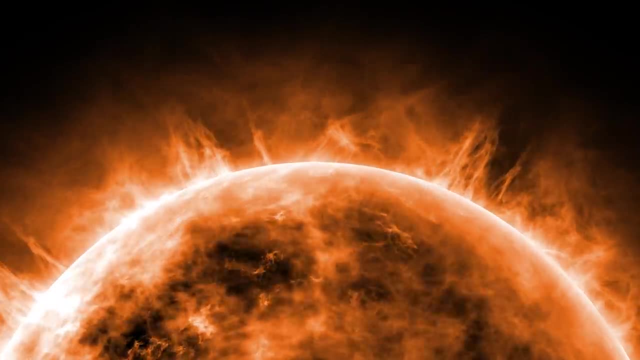 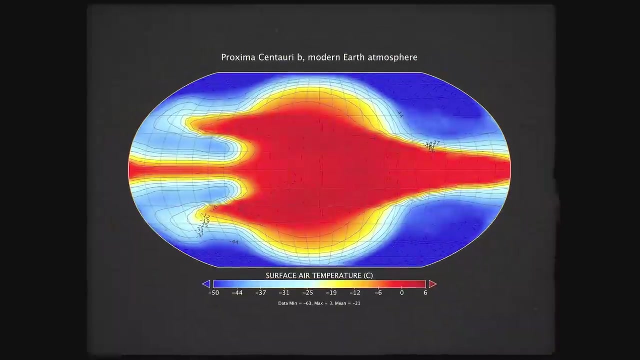 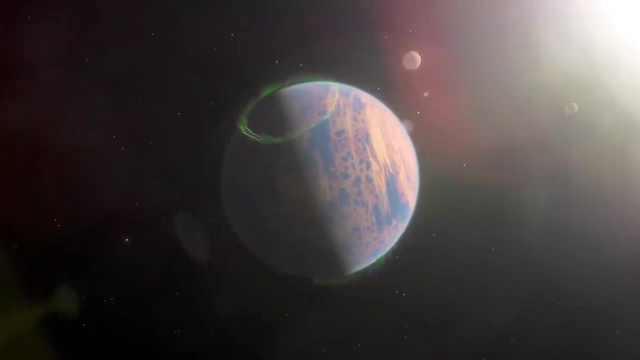 deep ocean from its surface. Right now it's uncertain whether a planet like Proxima B would be able to resist such damaging degrees of radiation, but models show that, with a thick enough atmosphere and a strong enough magnetosphere, it is at the very least possible. If so, the planet's magnetism would redirect the stellar winds to its poles, producing spectacular auroras many times greater in size and luminosity than those experienced by the Earth. This has all been to say that, while Proxima B certainly has some of the basic necessities of a planet like Proxima Centauri. 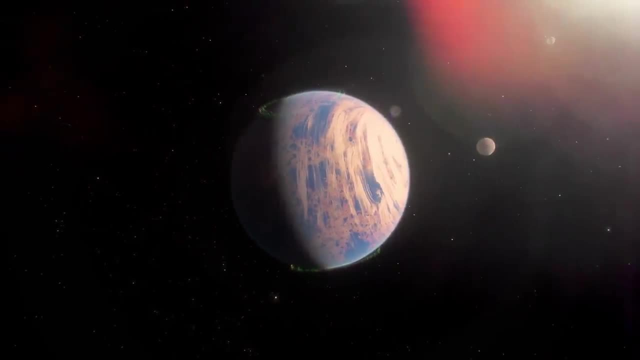 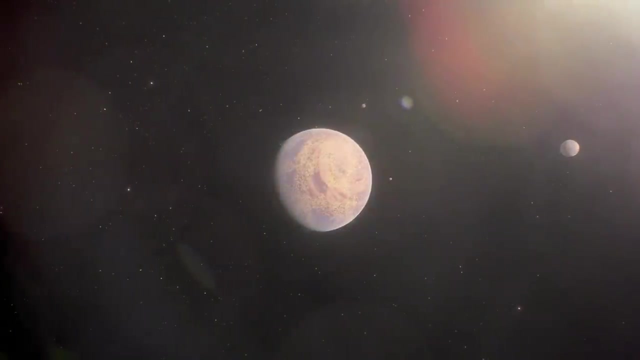 it's not just about the planet itself. it's about the planet itself as well. Proxima B is a planet that has so many of the necessities to support life. so many other factors go into this that, without more information, our image of the planet could range anywhere from. 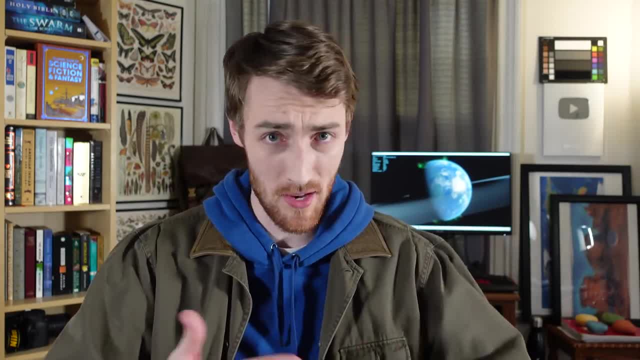 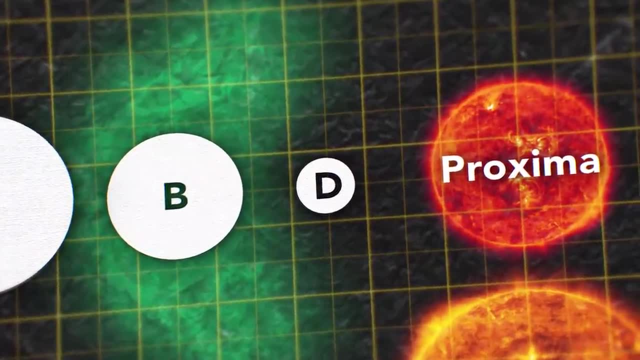 a dry and barren rock to a lush, wet world. But okay, I know what you guys are thinking. what about the other two planets discovered around Proxima Centauri? Well, despite what their names may lead you to think, Proxima D actually orbits closest to its star, With a mass of only around a 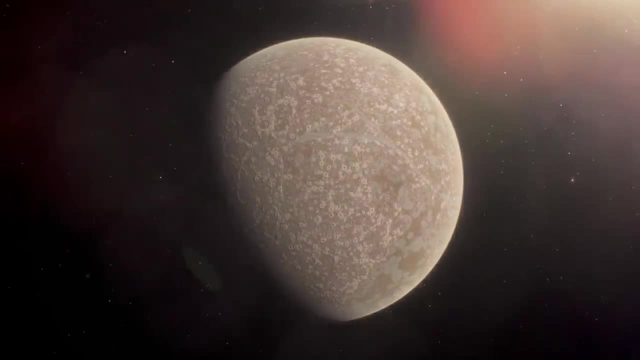 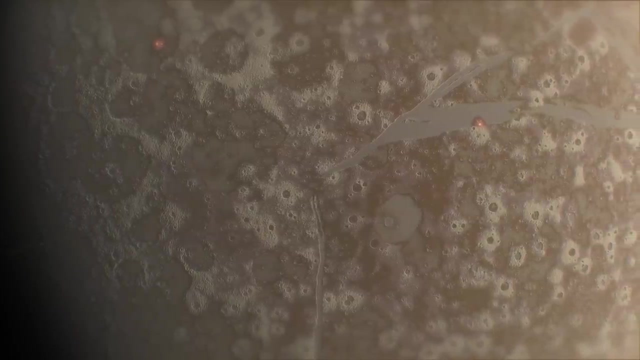 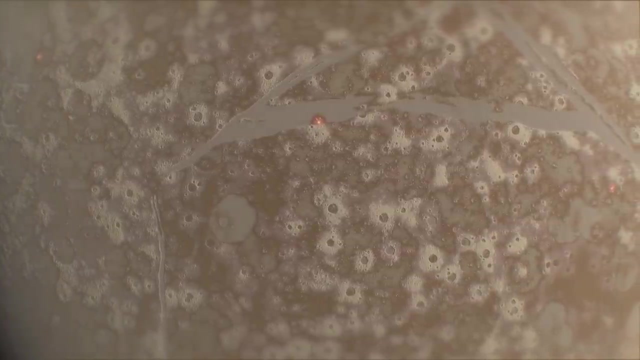 7 earths. Proxima D is one of the smallest exoplanets ever discovered, but also qualifies it as another rocky or terrestrial planet. That being said, at this short of a distance to its star, this will be a thoroughly scorched world, with a surface exposed to space and a poor candidate for 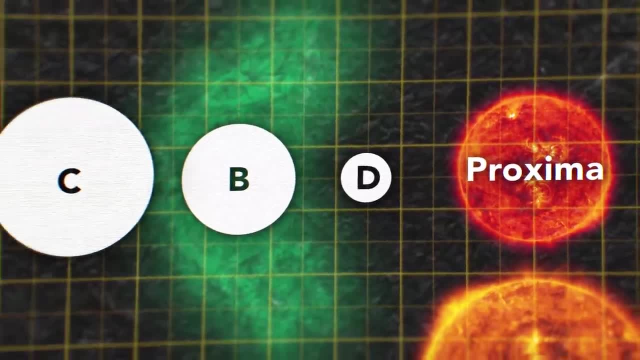 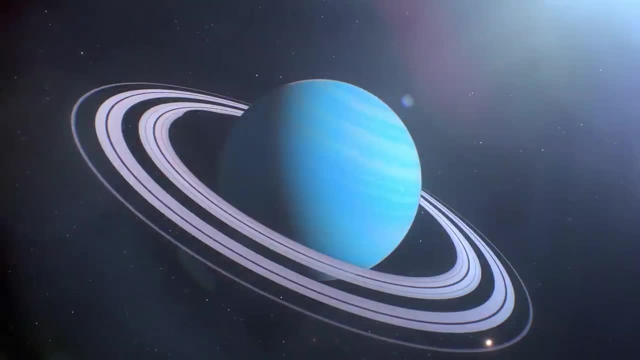 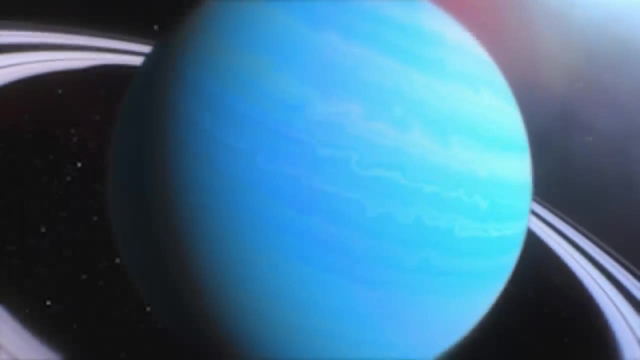 finding life. Proxima C, on the other hand, orbits the furthest away and, with a mass of around 7 earths, crosses the line from super earth into mini Neptune, plunging its surface beneath a dense, icy atmosphere Similar to the gas giants of our solar system. this is likely another. 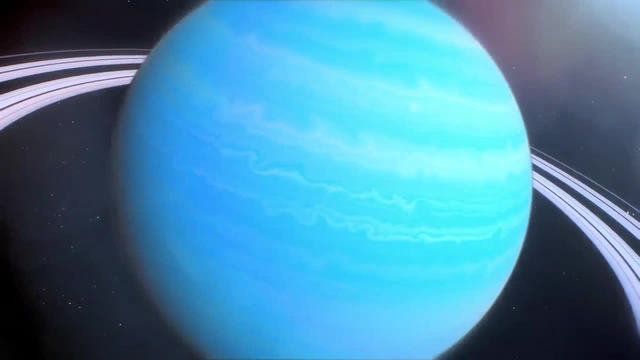 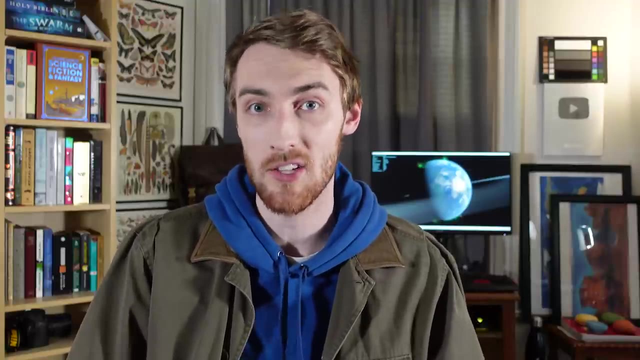 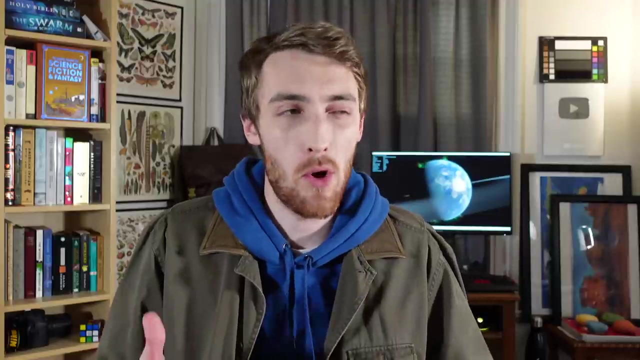 unremarkable world: cold, dim and lifeless. But we shouldn't forget that even planets like these could still become unexpected homes for biology, not in their clouds or on their surfaces, but rather among their many potential moons. And okay, while we technically haven't found even a single, 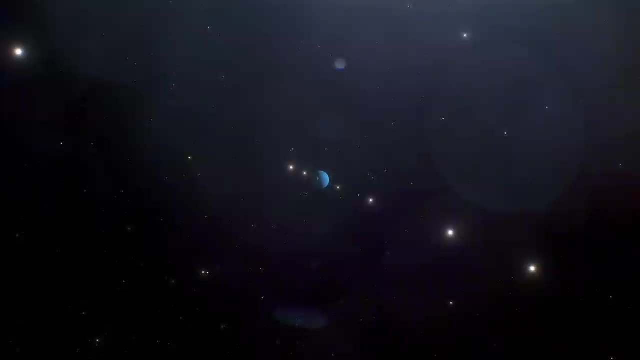 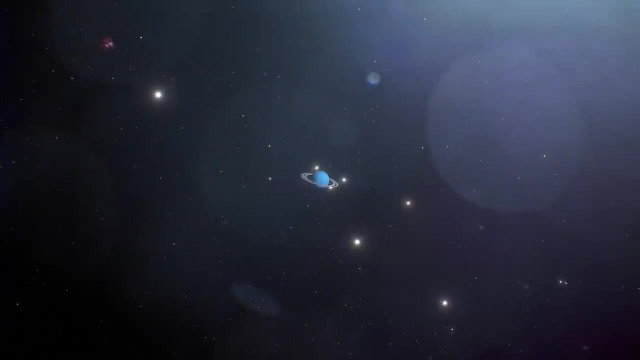 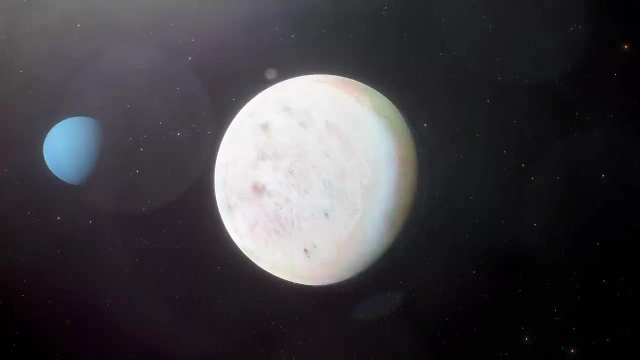 exo-moon. yet that doesn't mean there aren't, And if the mini-moons of our solar system's gas giants are any indication, chances are. planets like these will host several large satellites. Moons like Jupiter's Io, Saturn's Titan and Neptune's Triton show us that, even far beyond the 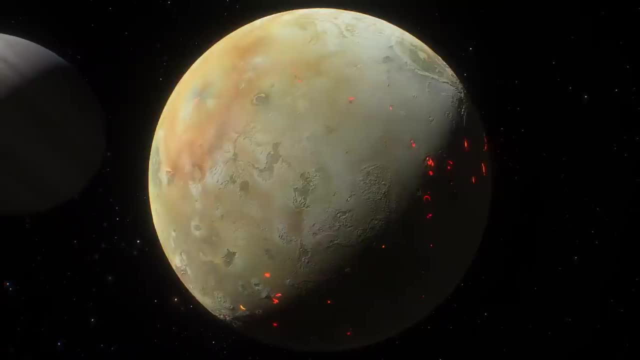 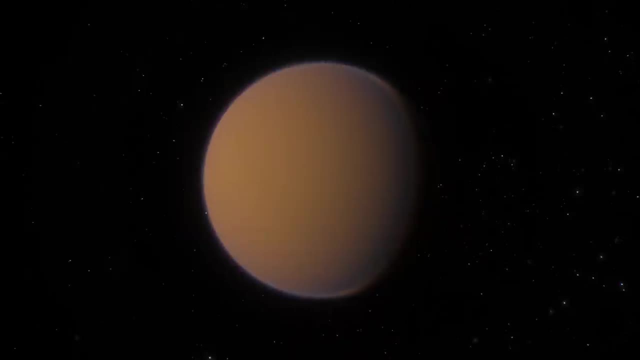 reaches of a star's supposed habitable zone. their interplay with their host planet's gravity can generate heat of its own enough to support substantial volcanism, build atmospheres, maintain liquid bodies and keep the planet warm. But that's not all there is to the exoplanets. 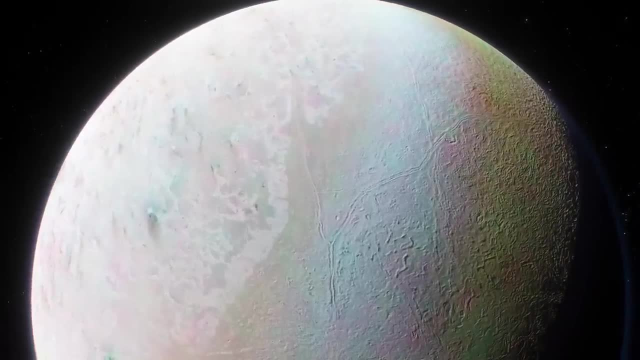 The exoplanets are all made up of the same kind of solar system. They are also large and they are a part of an aerodynamic system. They can even harbor entire subsurface oceans. This endless possibility for exomoons in turn means that even planets like Proxima C 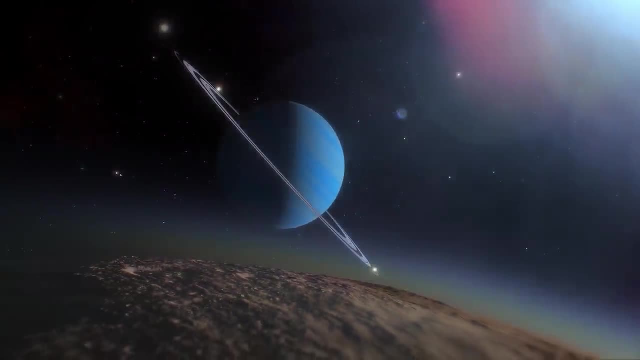 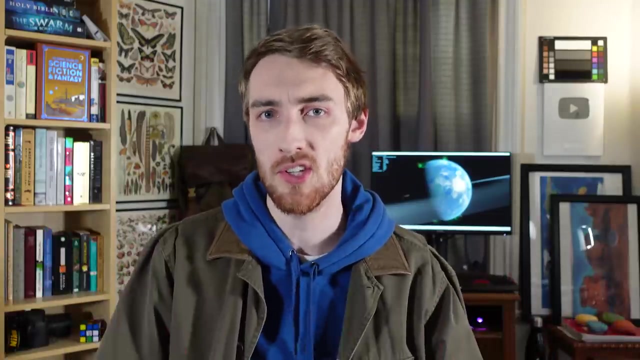 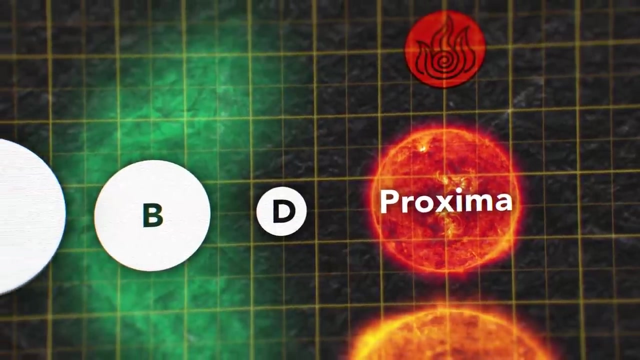 that would otherwise be written off as too big or too cold should not be so quickly dismissed as potential alien habitats. Overall, the Proxima system represents an almost perfect example of a typical or standard planetary system: A dim star parent to one small rocky planet. it is typically a star. with an orbit of 12 to one-third of its size. Rather than being a star of a single planet, it is a star that is not related to any other planet. A star that is not related to any other planet or an asteroid or any other planet, But it is a star that is not related to any other planet. 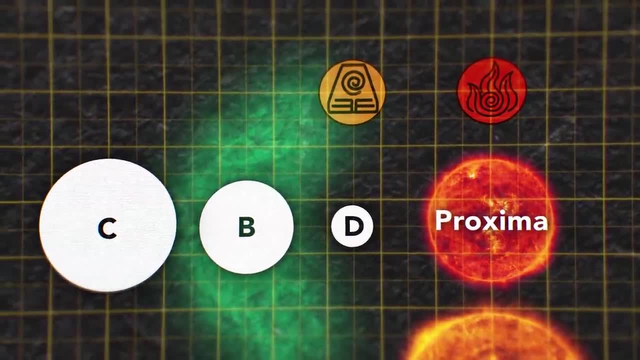 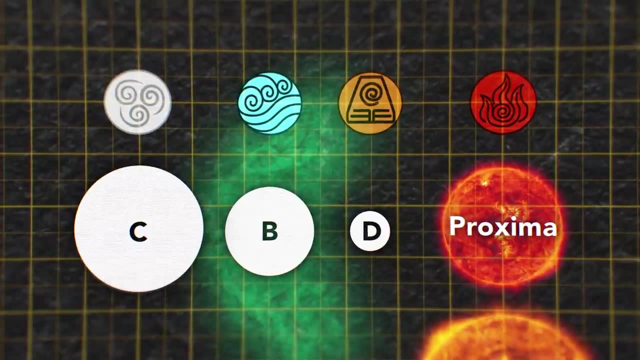 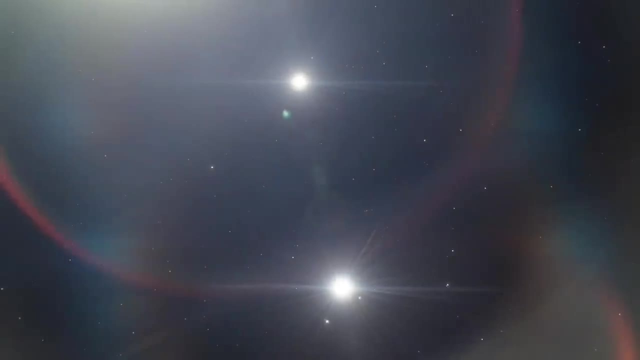 parent to one small rocky planet, one medium-sized, potentially wet planet, and then one big gaseous one appearing almost like a simplified version of our solar system. As for the other two stars in Alpha Centauri, well, we don't know. I mean, we know it's possible for there to be planets. 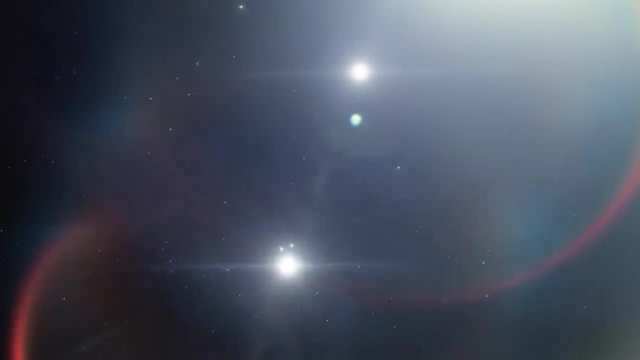 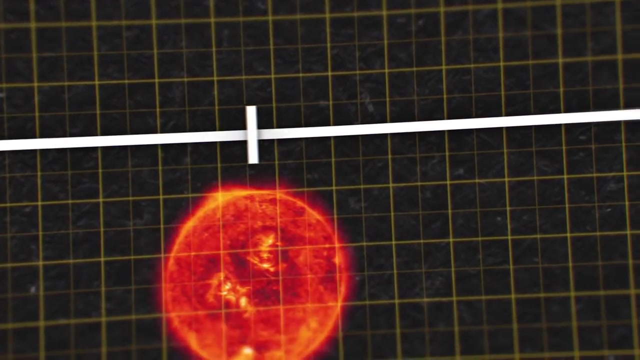 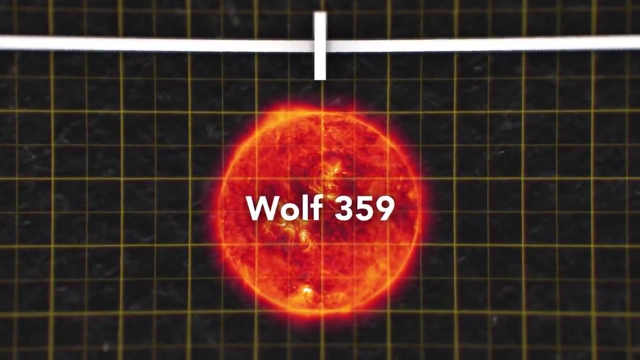 orbiting either one or even both of these stars, but so far none have been confirmed. Continuing our trek through space, the next closest star to have confirmed exoplanets orbiting it would be Wolf 359,, at just eight light-years away, another red dwarf too dim to be seen from Earth, Which is 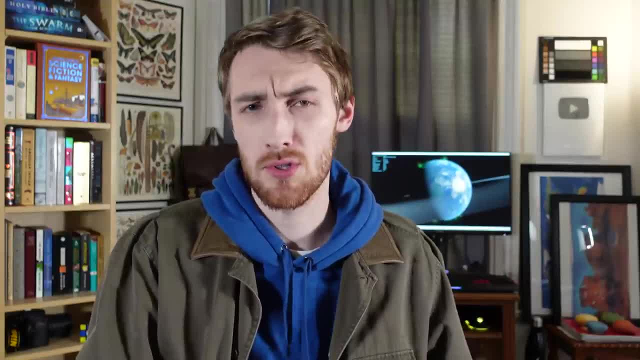 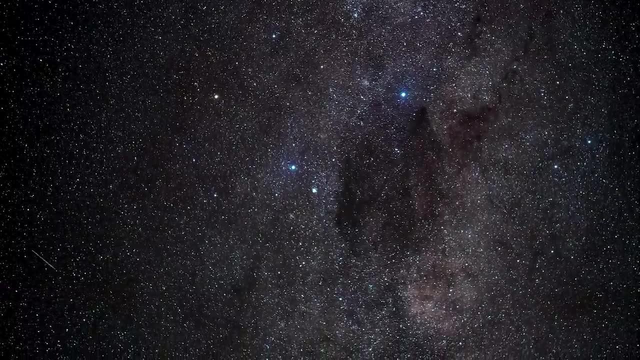 sort of weird, when you think about it, how most stars closest to us are literally invisible, while others can actually turn out to be more than one star, and serves as a good lesson on just how much remains to be discovered across the vastness that is space Following in the same. train of thought, we're going to be able to find out how many stars there are in our solar system. Following in the same train of thought, we're going to be able to find out how many stars there are in our solar system. Following in the same train of thought, we're going to be able to find out how many stars there are in our solar system. As the proximas. the Wolf 359 system features one close-orbiting rocky planet creatively named Wolf 359c, and another more distant gaseous planet, Wolf 359b. Wolf 359c, the smaller terrestrial planet, orbits far too close to ever be considered. 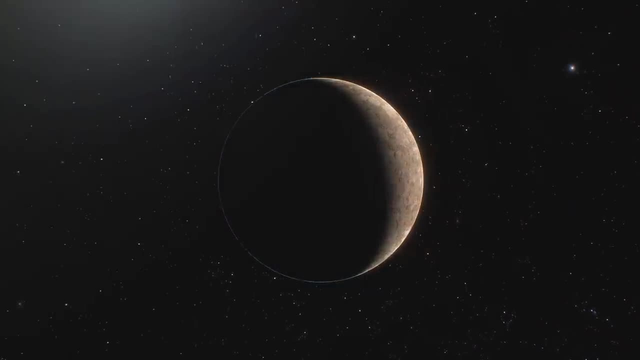 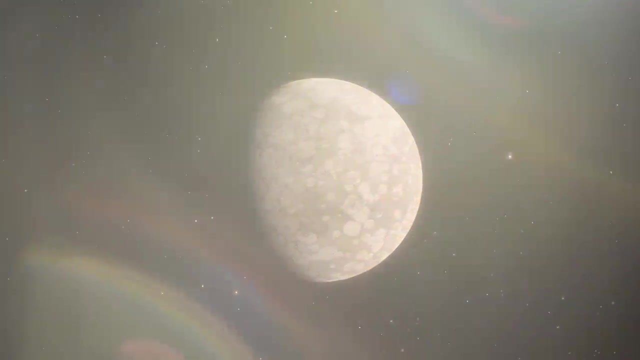 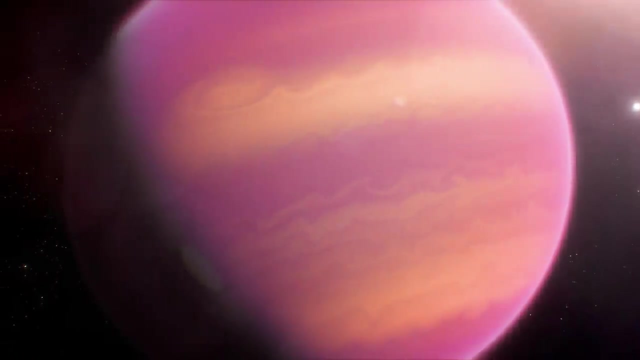 habitable, receiving over three times more radiation from its star than the Earth receives, likely stripping its surface of any atmosphere, leaving it as a barren rock comparable to Mercury. In contrast, at over 40 Earth masses, Wolf 359b is definitely a gas giant. 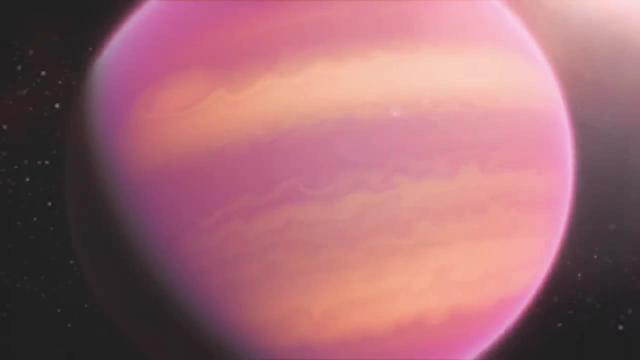 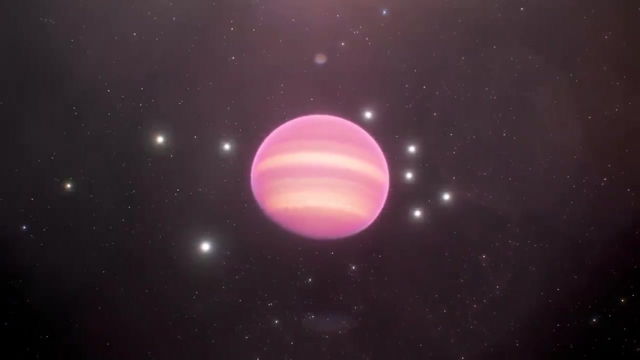 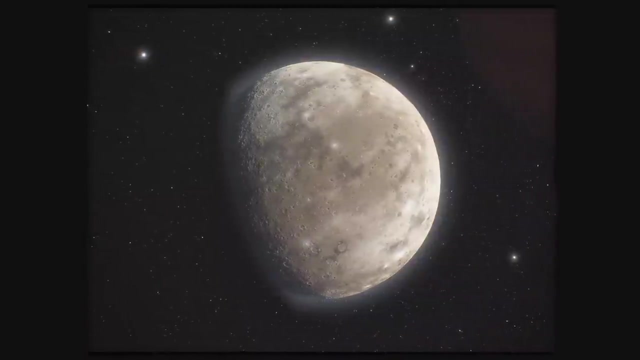 sitting between Neptune and Saturn. in terms of size, With an even greater mass than Proxima c, not only does Wolf's likelihood of hosting moons increase, but so does the number of moons it's capable of hosting. If we think of each exomoon as a roll of dice, then the more you have, the more likely it is that at least one 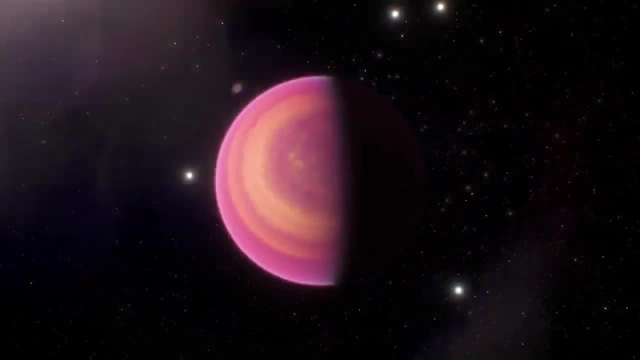 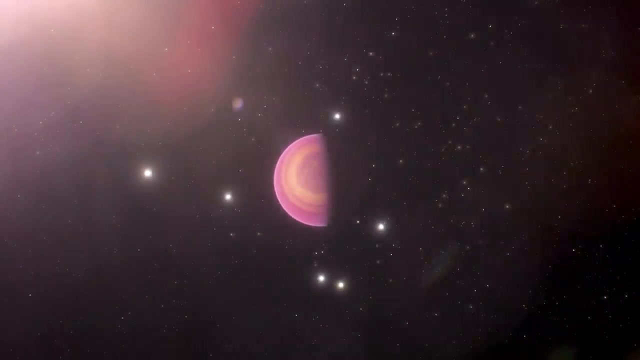 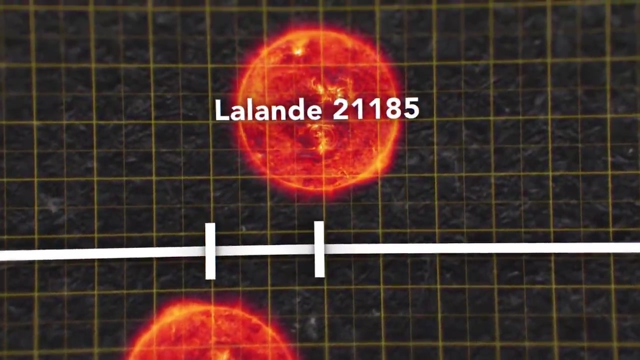 one has favorable conditions, and so, as we continue to explore space, I wouldn't be surprised if we found an interesting correlation between a gas giant's size and its probability of harboring life. The next closest exoplanets can be found around the star Lalande 21185, yet another red dwarf. 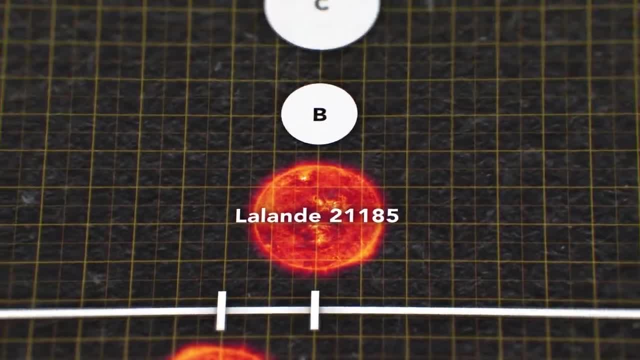 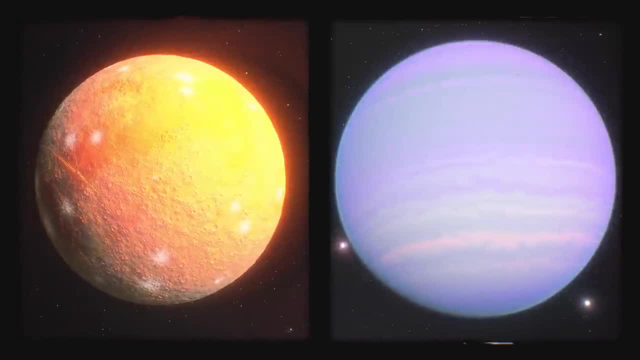 too faint to be seen from the Earth, where we'll find a very similar situation as Wolf 359, two confirmed exoplanets, one small rock and one big ball of gas, While Lalande B is only twice as massive as the Earth, suggesting a similar size and composition. 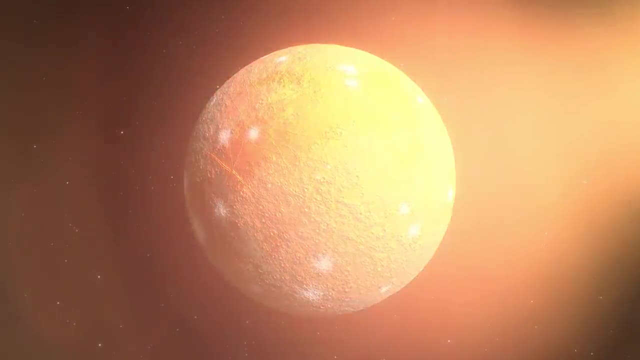 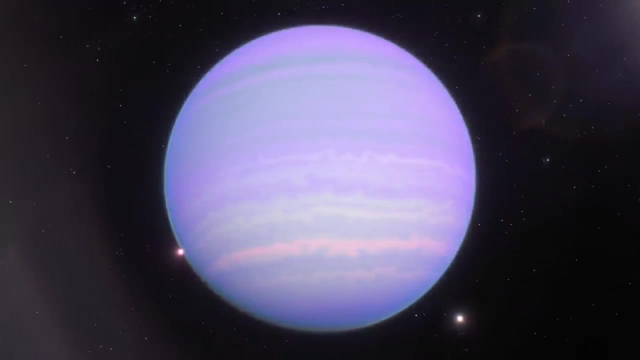 it again orbits far too close to a flare star to be considered a prospect for life. and Lalande C is another mini-Neptune equally uninviting to biology. And it's by this point that I hope you're picking up on a pattern. 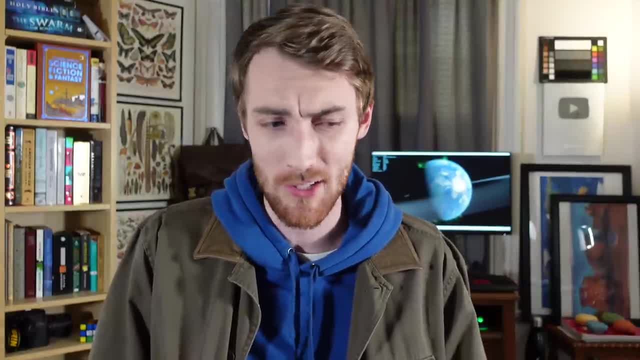 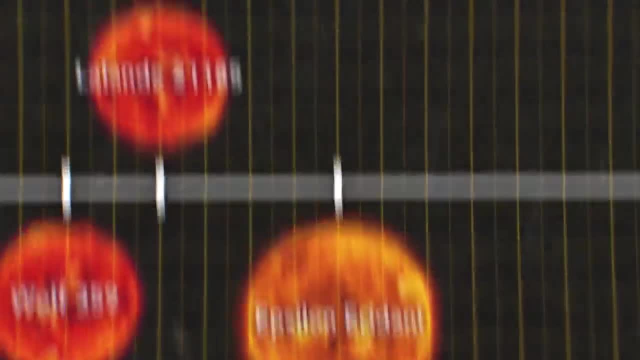 As it turns out, habitable planets are a little hard to find, And so, if you want to see some more promising outlooks, we're going to have to speed through a few of these. Next up is Epsilon Eridani, a K-type star that falls between the size of M-type red. 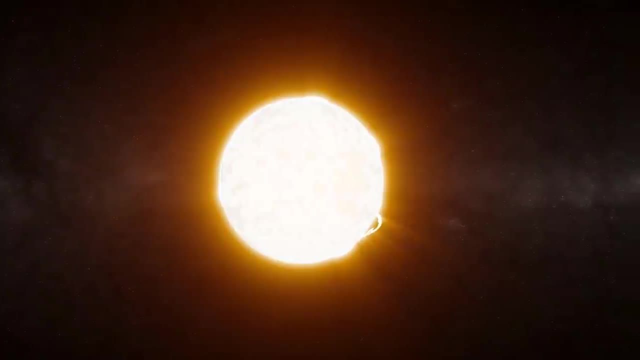 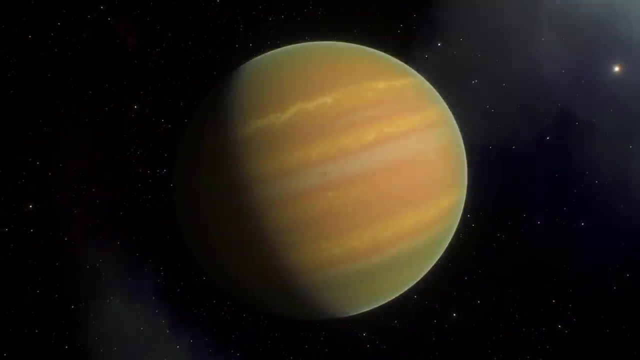 dwarfs and G-type stars like our Sun. These are also known as orange dwarfs, and this one is known to host only a single planet At a mass of approximately 1.2 Jupiters. this is definitely another gas giant, and 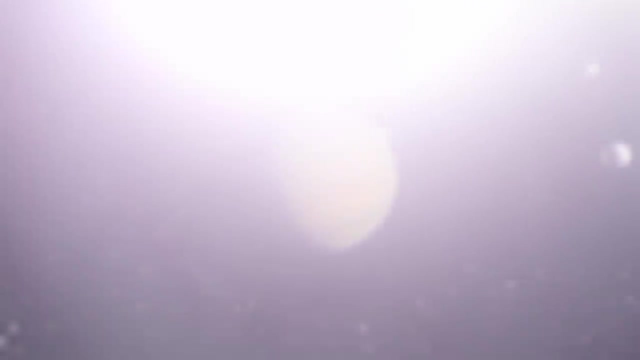 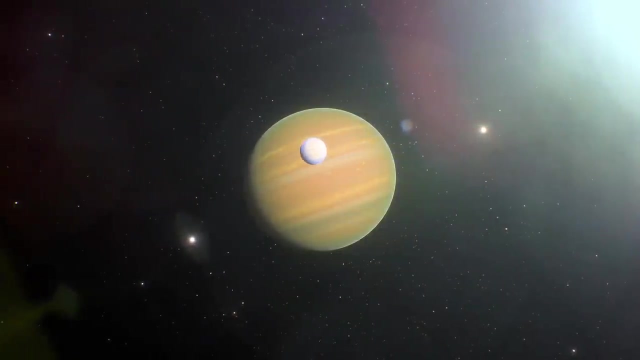 the biggest one we've looked at so far. Besides its many possible moons, the only notable quality of this Jovian world is that it's the first and only one we'll look at today that's been given a proper name: Aegir. 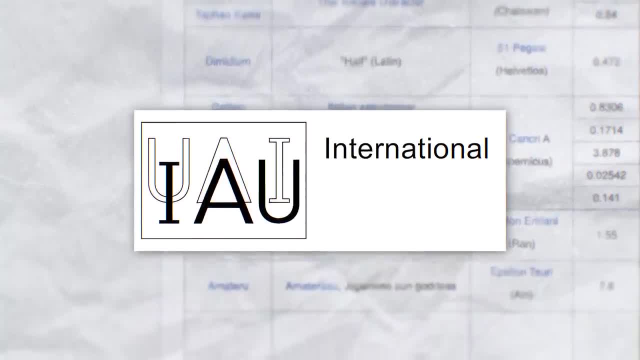 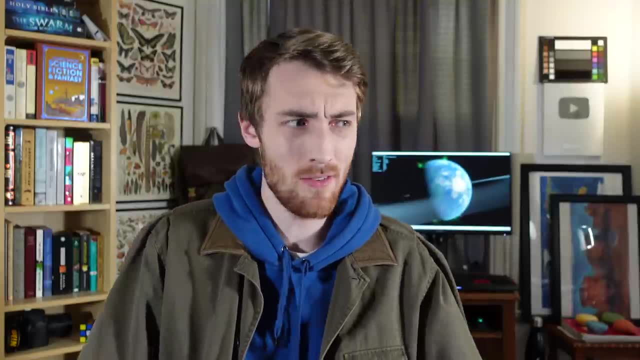 This name comes from contests held by the International Astronomical Union in 2014 and again in 2019, though, to be honest, I couldn't find any rhyme or reason behind the planets they chose to receive names. Some were big, Some were small. 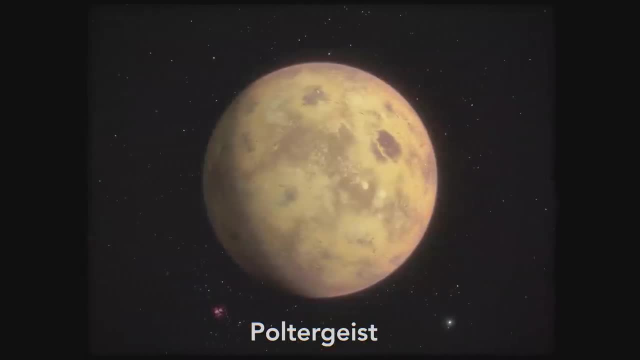 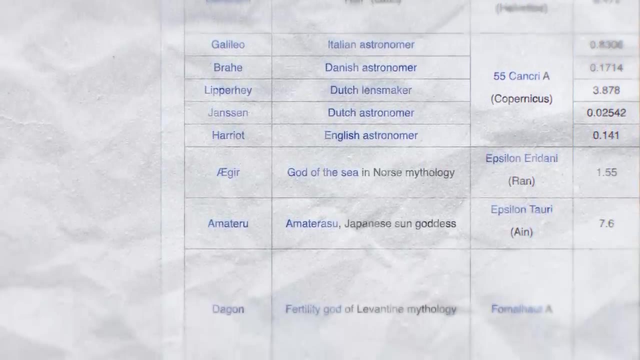 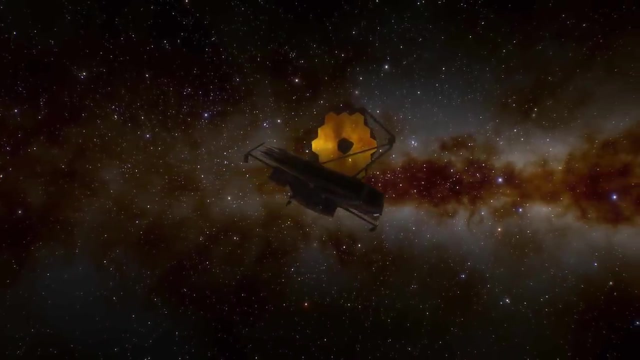 Some were nearby, Others were incredibly far away. Some could maybe host life, Many more, like Aegir definitely could not, And all around. as it stands now, it's a pretty mixed bag when it comes to named exoplanets, But I expect that as the first images of the nearest alien worlds start coming in through, 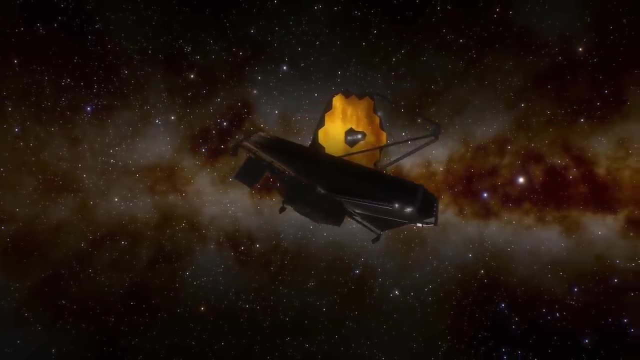 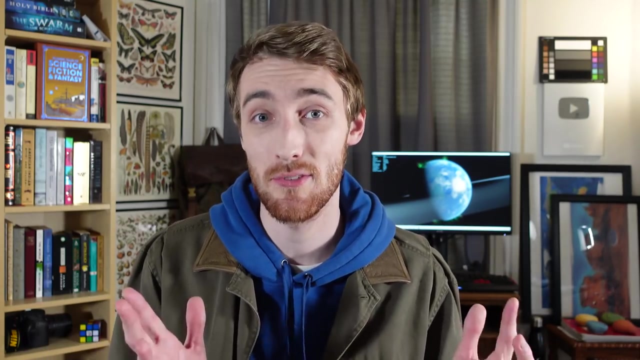 the James Webb Space Telescope and intense scientific analysis begins, it'll be these planets that are prioritized for proper titles, Meaning even the names you're hearing in this video will probably be the names of these planets, And this video will probably sound incredibly outdated sooner rather than later. 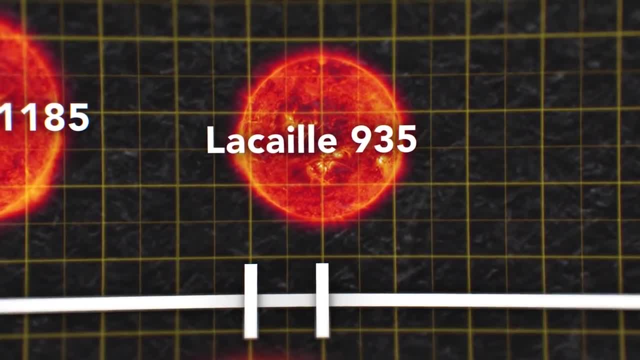 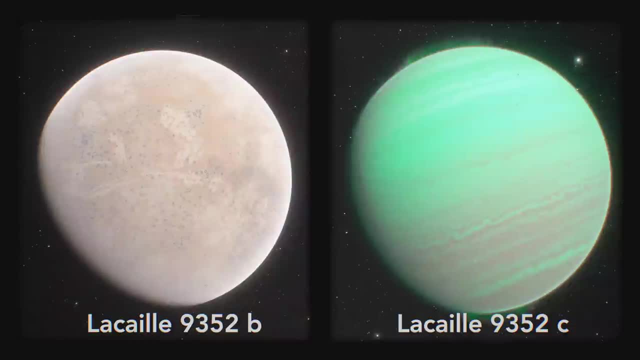 Continuing on, next we'll come across LaSalle 9352.. But okay, to avoid things getting repetitive, it should suffice to say that neither of LaSalle's two planets appear to orbit within the habitable zone, So we can probably just skip them for now. 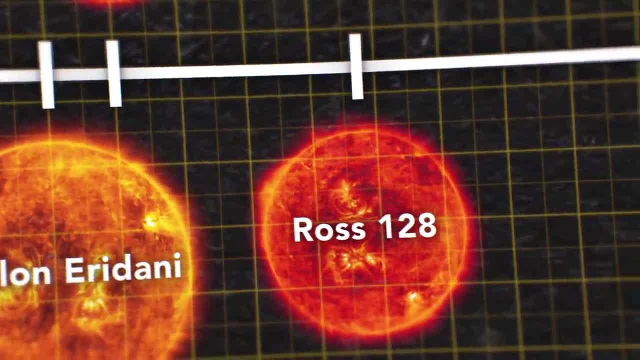 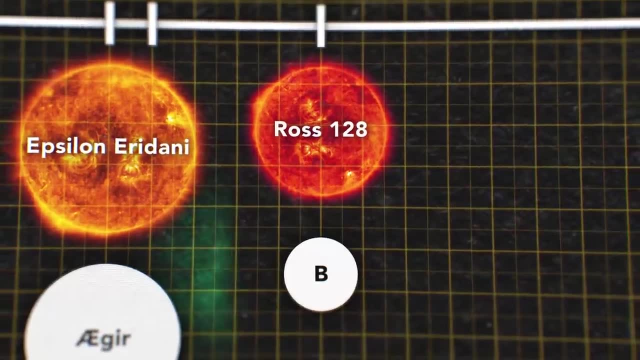 And okay. finally, this brings us to the star Ross 128, found at a distance of 11 light years away. While only one planet has been confirmed here, this is nonetheless where we'll find the planet we're looking for. Nonetheless where we'll find perhaps the most promising prospect for life so far, though. 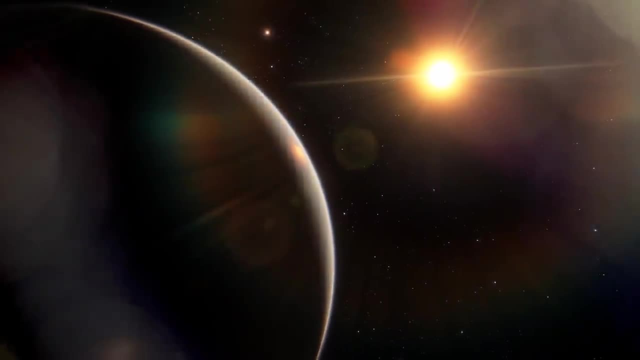 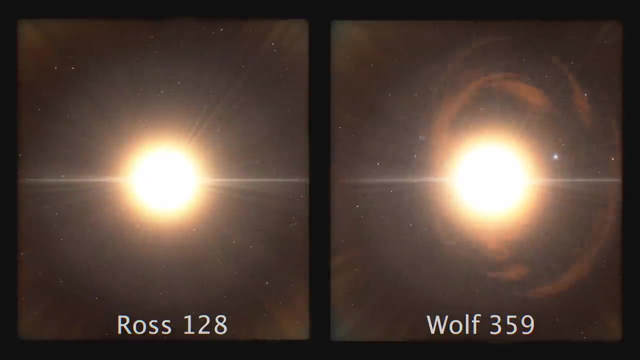 much of this isn't due to the planet itself, but rather the star it orbits. While sure it's another red dwarf, the major difference here is that Ross 128 is a relatively quiet star, producing far less damaging radiation than the others we've looked at today, giving 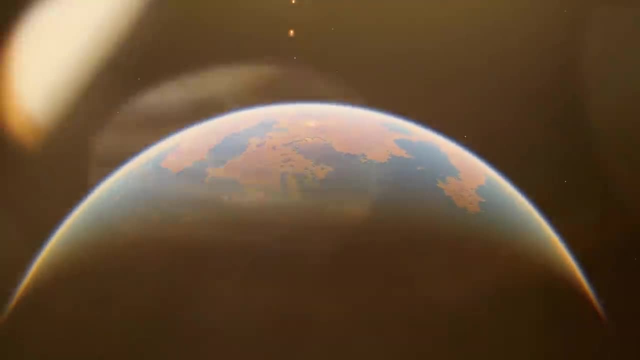 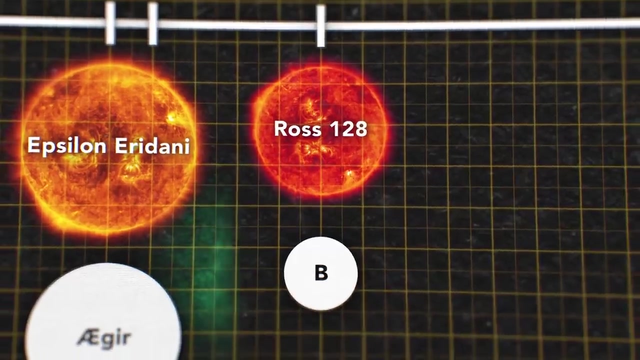 Ross 128b more than a good chance of supporting an atmosphere With a mass of 1.8 Earths. this is likely another 2.8 Earths, But that's not all. This is likely another terrestrial world, one that orbits on the inner side of its habitable. 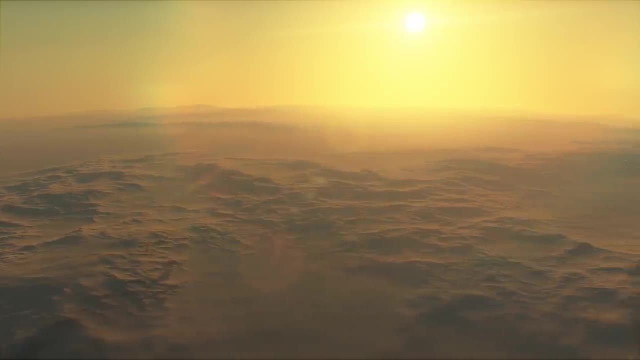 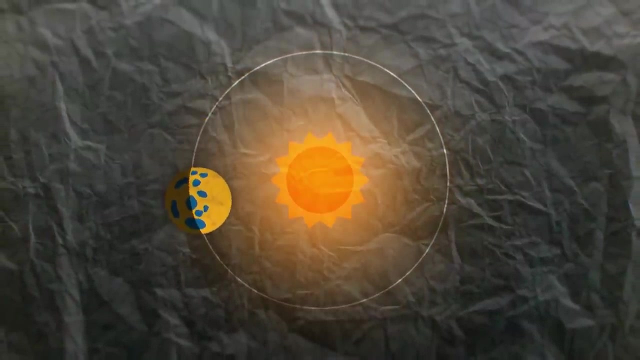 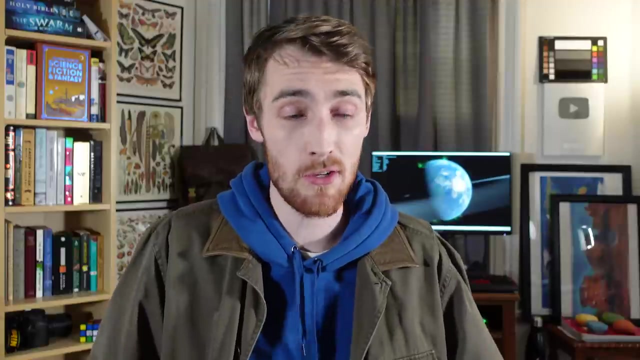 zone, making this surely a hot environment. This closeness also means the planet has a high likelihood of being tidally locked permanently, exposing one side of its surface towards its star and the other towards the black void of space. This, however, appears to be the norm among planets orbiting red dwarfs, including all. 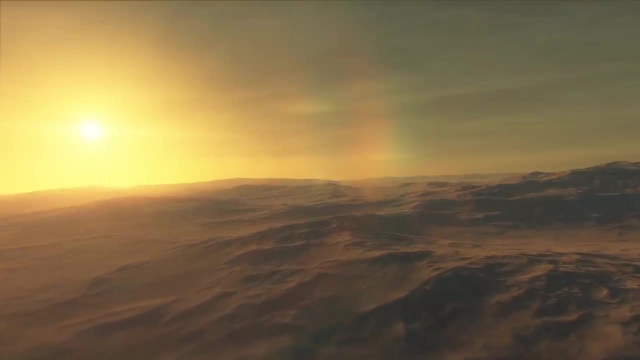 the others mentioned so far. While not necessarily a death threat, the planet's orbit is likely to be closed off and the planet's orbit is likely to be closed off, and the planet's orbit is likely to be closed off and the planet's orbit is likely to be closed off. 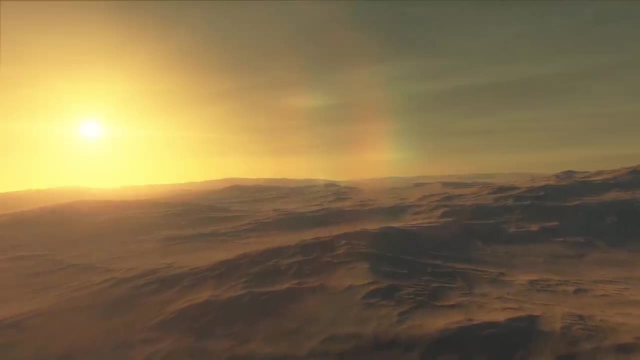 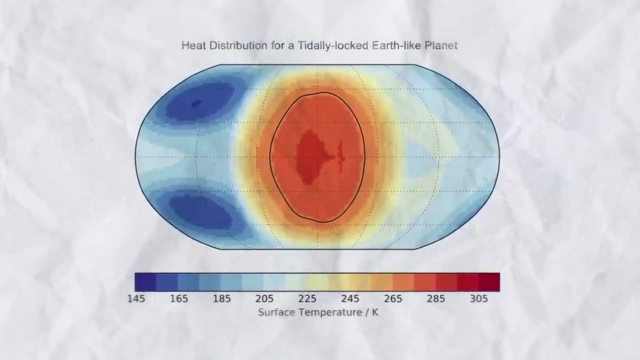 In a math sentence. it sure would make life in a place like this more complicated, though current models do show that with an Earth-like atmosphere, the temperature extremes between the hot and cold sides wouldn't be so drastic as to make the whole planet uninhabitable. 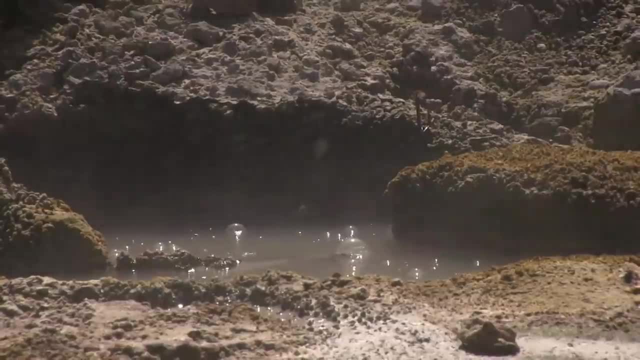 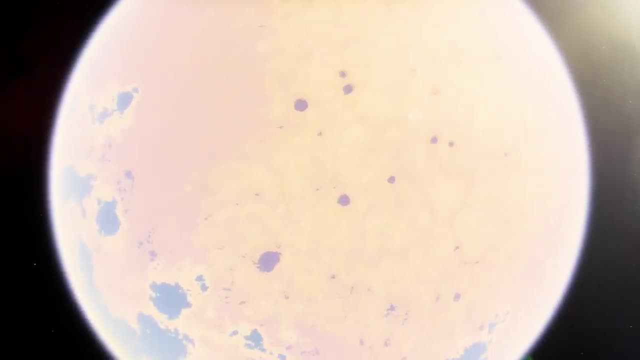 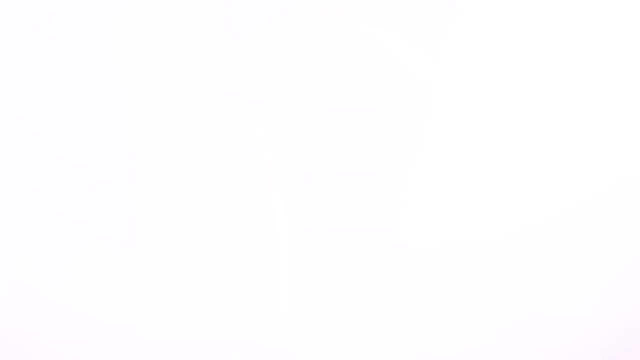 Of course, that still doesn't mean life here would be easy. Being a hot world, it's possible. temperatures under the focus could reach high enough to spontaneously boil water, leaving a vast desert wasteland at its center, surrounded by a rank of warm lakes where the sunlight isn't so intense. 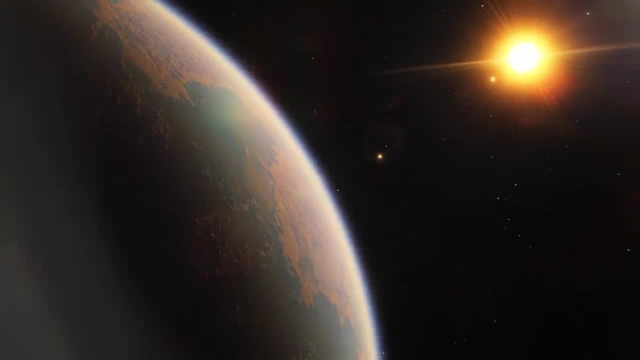 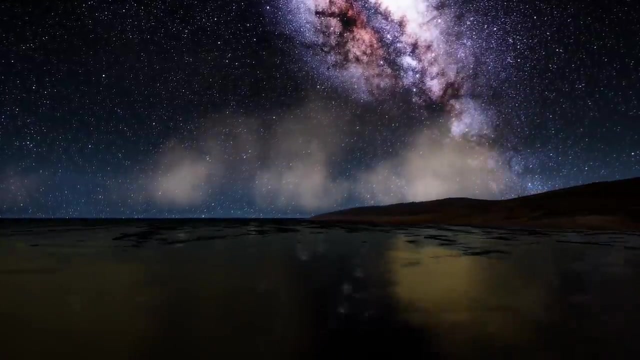 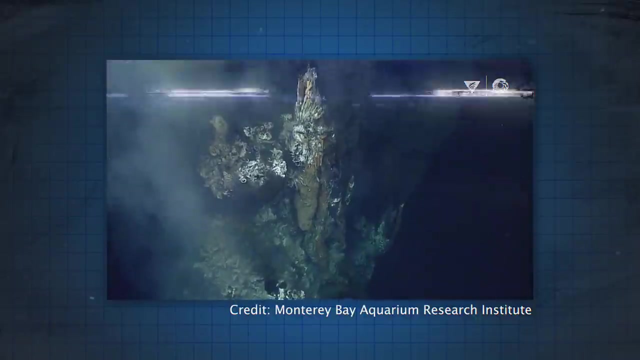 Beyond this twilight region. if the planet contained enough water, it's possible that oceans could cover its backside. These would be night oceans, places that never see daylight, where the stars serve as the only illumination, But if exploration efforts of our own oceans' depths have taught us anything, it's that. 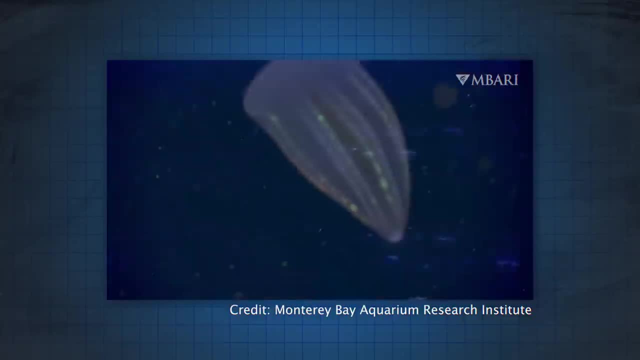 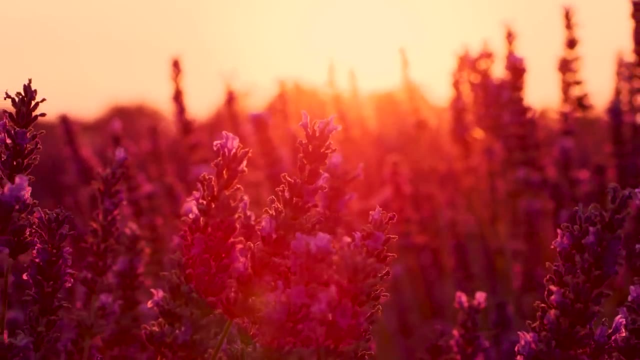 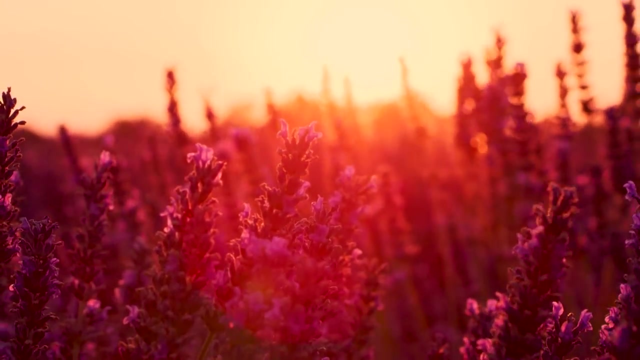 life doesn't always need light, and places such as this could easily be rich with all sorts of fantastic things To better control the amount of light they receive from their star. any plants that do manage to photosynthesize in the narrow twilight zone would also likely be red rather than. 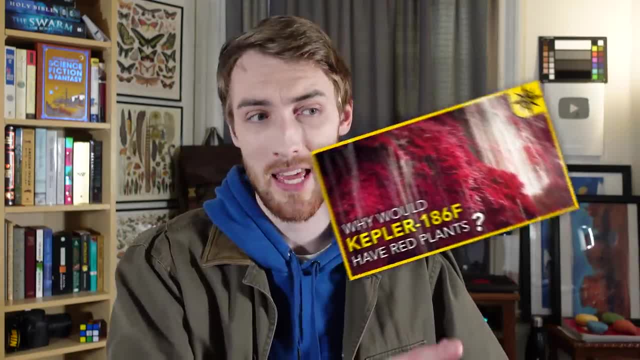 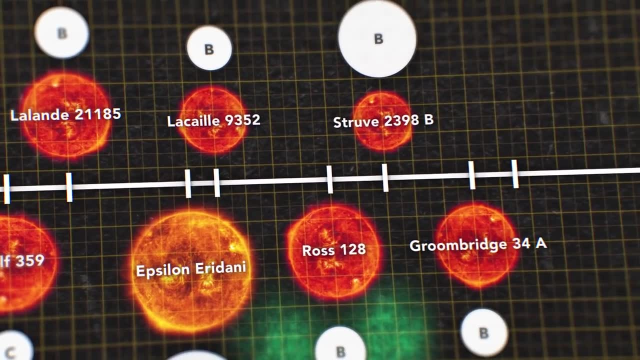 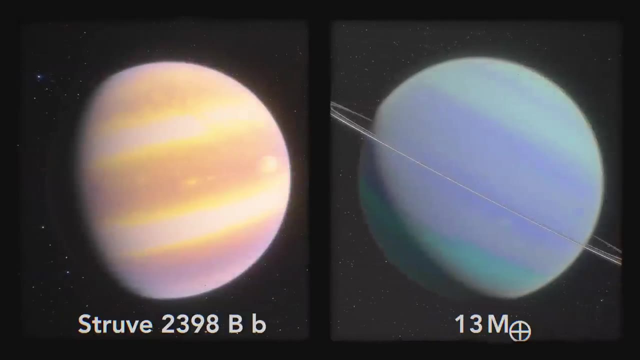 green, Though actually I already spent a whole other video explaining how this all works, so if you're curious, go check out that video. next, Leaving Ross 128 will reach another patch of mostly uninteresting sights. Struve 2398's: two planets come in at 13 Earth masses. 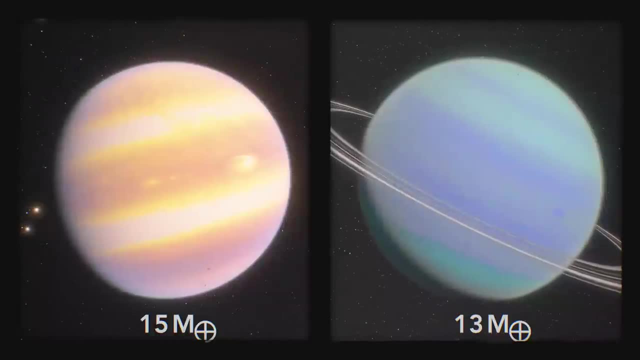 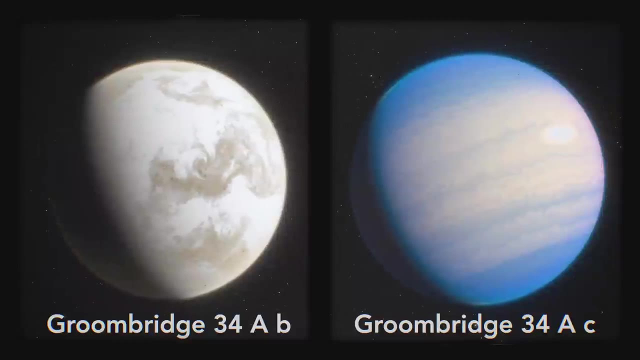 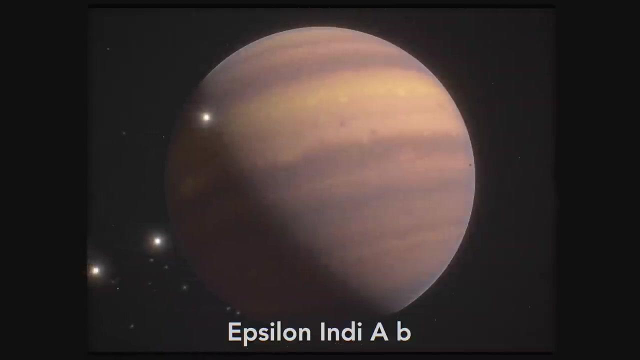 And 15 Earth masses, making them both likely Neptune-type ice giants. Groombridge 34's two planets are a familiar rock and gas pair where both lie outside the habitable zone, And Epsilon Indi's single planet is three times more massive than Jupiter, qualifying. 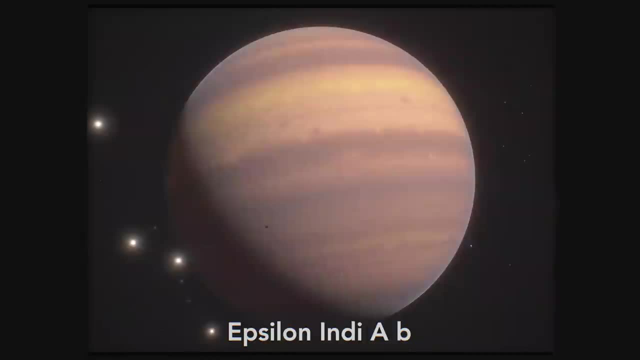 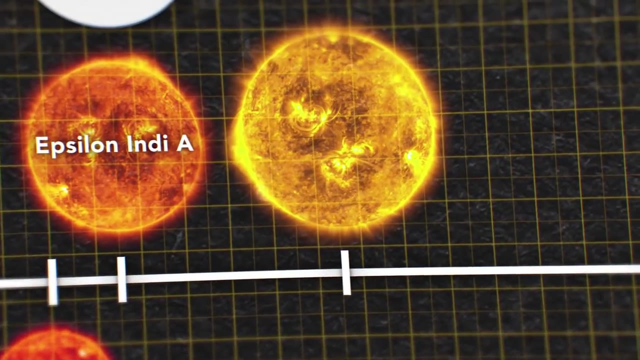 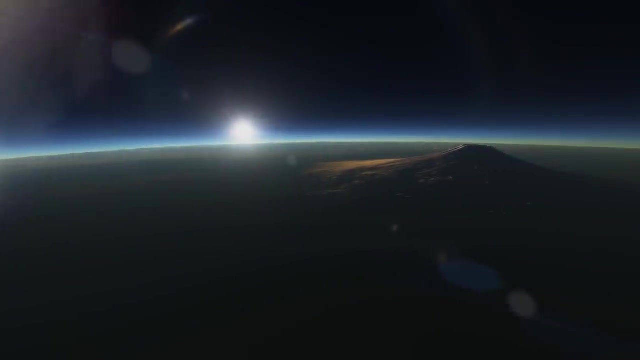 it as definitely uninhabitable, though again, perhaps harboring hundreds of prospective moons. But once we've ventured 12 light years away, we'll arrive at our next point, Tau Ceti. For a nice change of pace, Tau Ceti is not another red dwarf, but rather a G-type star. 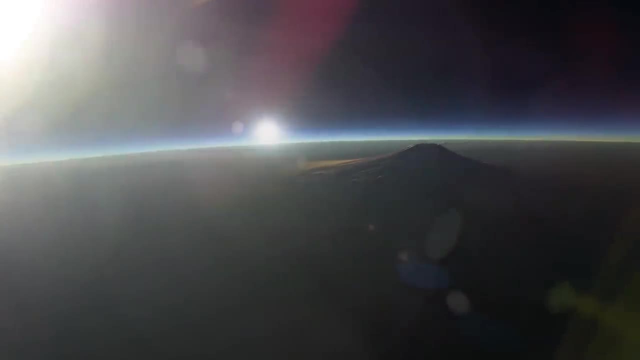 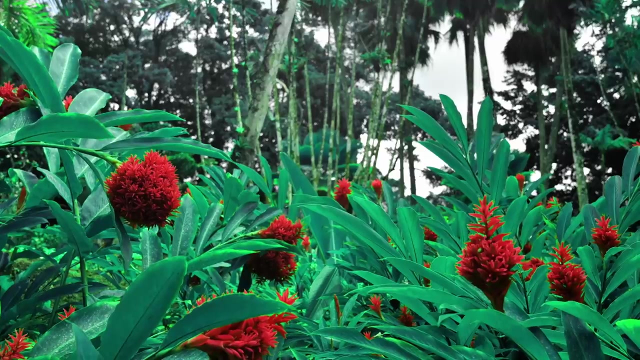 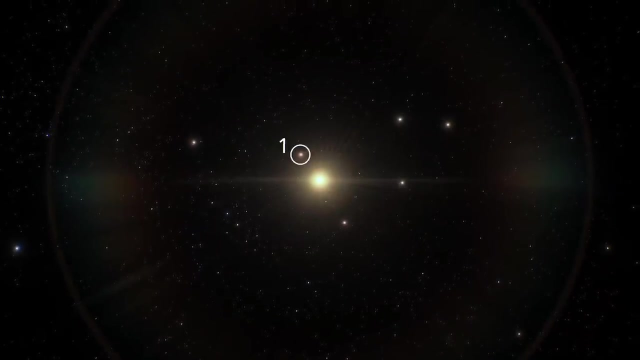 like our Sun, with a similar size, luminosity, temperature, even color, meaning. any plants here would most likely be some shade of green, though not necessarily the same exact green as we're familiar with. The similarities continue when counting the planets found in the system where 1,, 2,, 3,. 4 confirmed and 4 additional unconfirmed. So that's the point: The unconfirmed planets add up to a potential 8-Planet system. For now, though, I'm only going to look at the 4 planets that have actually been proven. 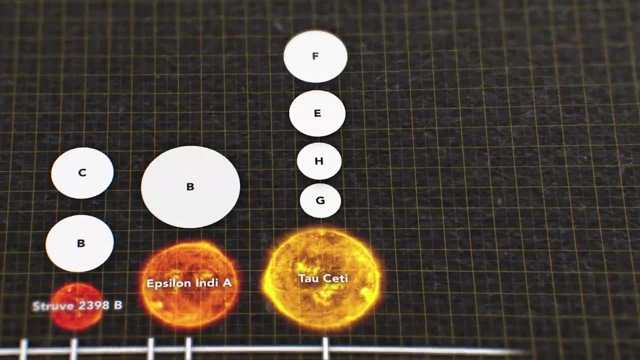 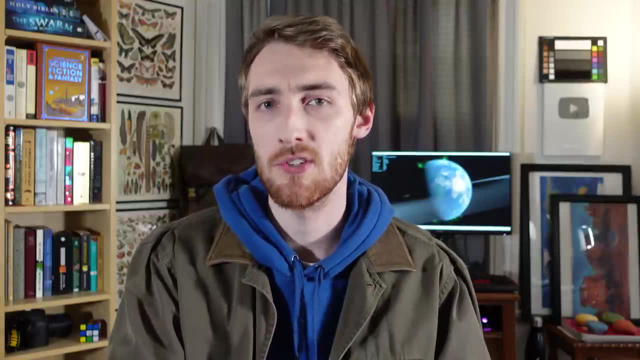 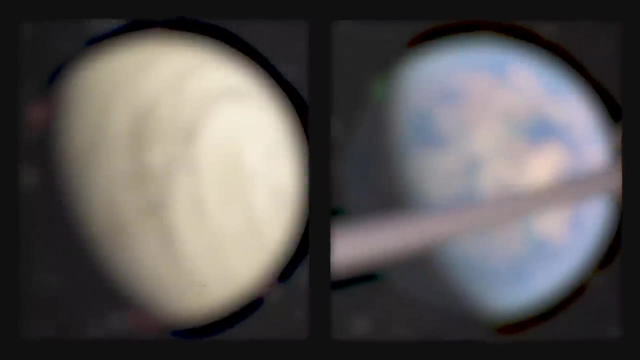 Tau Ceti G, H, E and F. Two of these Tau Ceti E and F orbit on either side of their habitable zone. The difficult thing about these two planets, however, is that only their minimum masses are known, both being at least 4 Earth masses. This is important to know because anywhere over 5 Earth masses are known and they're known to be a minimum mass. This is important to know because anywhere over 5 Earth masses are known. This is important to know because anywhere over 5 Earth masses are known and they're. 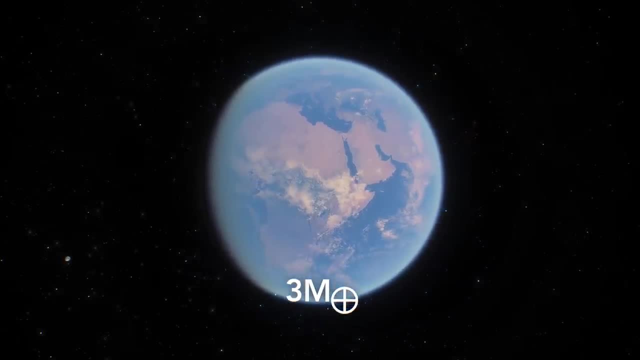 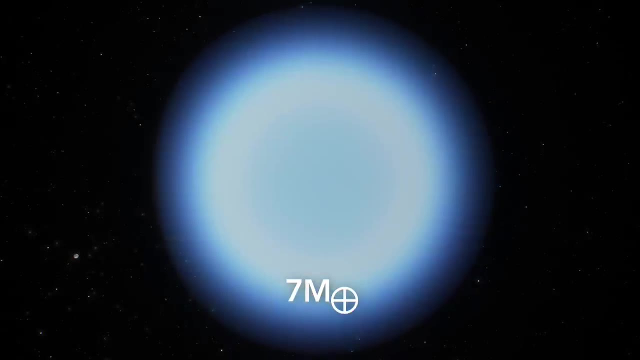 known to be a minimum mass. Earth masses and a planet runs the risk of becoming a mini-Neptune, where their gravity can hold on to such a dense atmosphere that its surface plunges into obscurity beneath heavy clouds of ice. Four Earth masses puts these planets in. 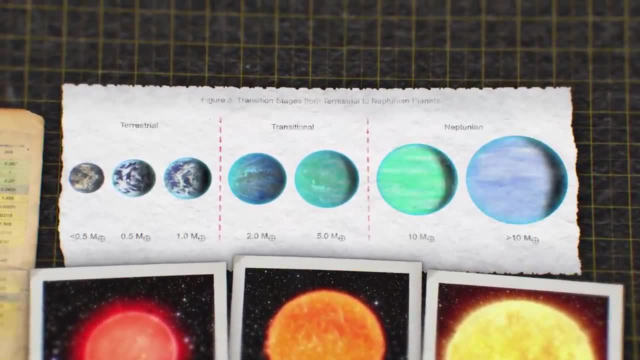 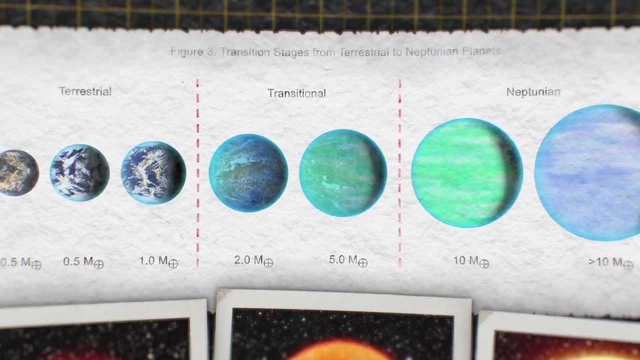 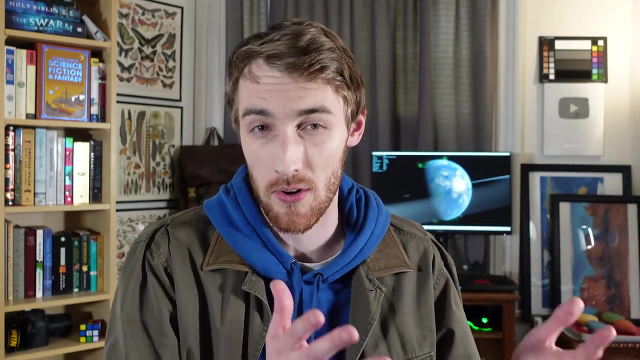 the gray zone between terrestrial and Neptunian, meaning if either of their masses turn out to be any greater than this lowest possible estimate, then they're likely not worth talking about. But if we put on our optimist hats for a minute and just believe that these planets aren't too far gone, then we'd 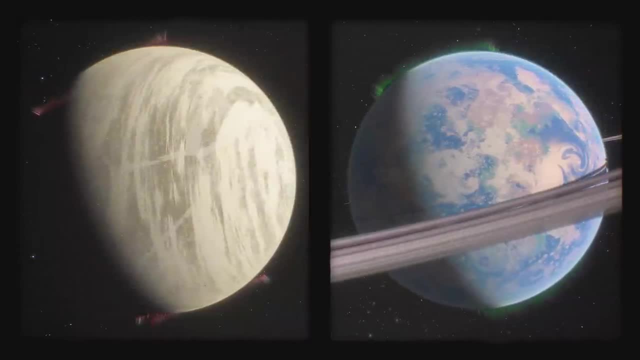 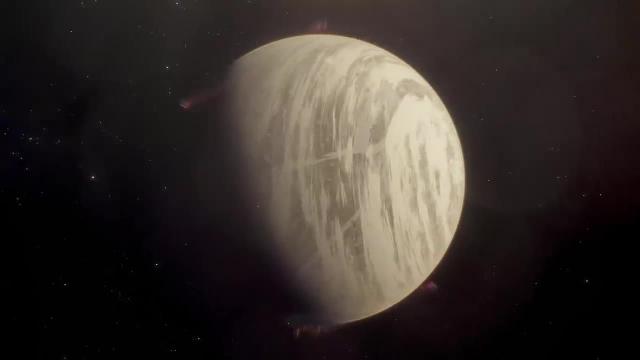 find two super-Earths featuring thick atmospheres, strong magnetospheres and lots of volcanic activity. For Tau Ceti E, however, the closer of the two, this bigger size, would likely be a death sentence, its atmosphere trapping far too. 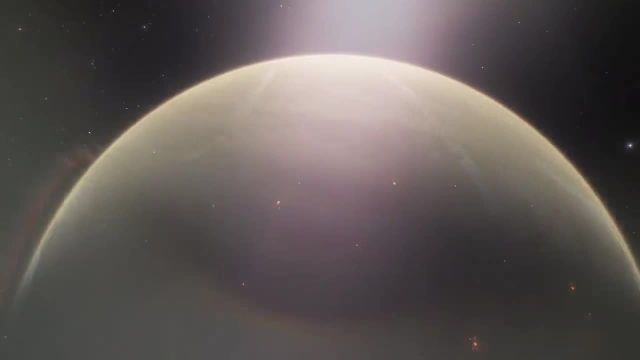 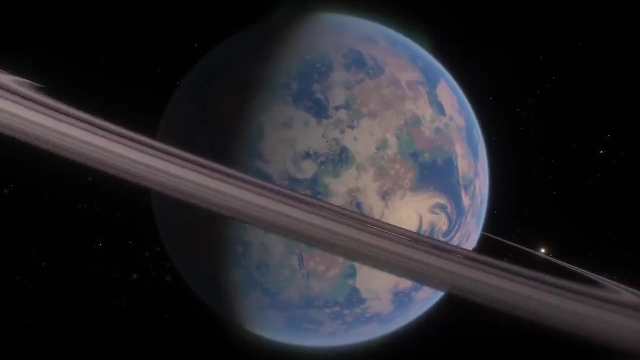 much of the Sun's energy to be habitable, generating a runaway greenhouse effect that lead it to resemble Venus more than Earth. On the other hand, being on the far side of the habitable zone, Tau Ceti F's great size would be a blessing, as its 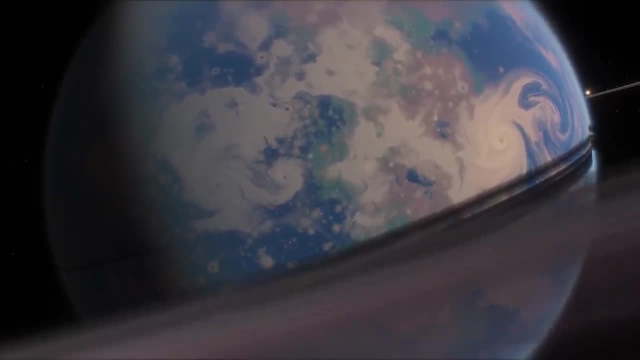 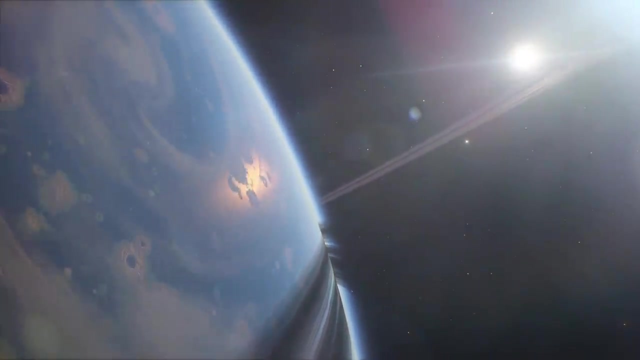 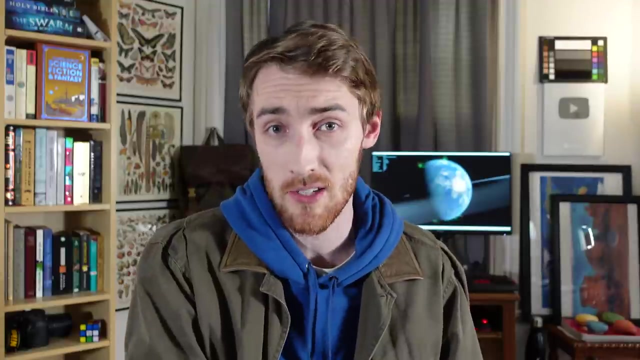 thicker atmosphere would allow it to more effectively trap what little heat energy reaches its surface, helping it fight against the cold of space and increasing its potential habitability. Of course, this doesn't mean life is definitely here, only that one of the many necessary factors is satisfied. a 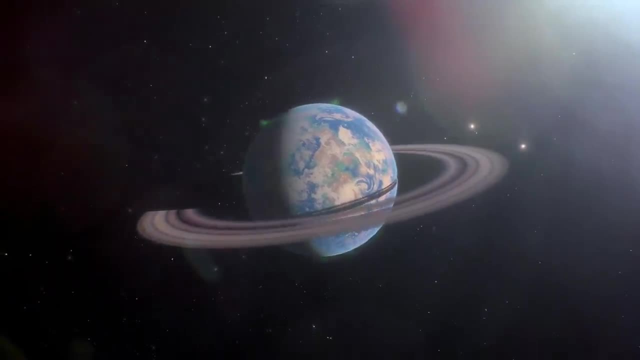 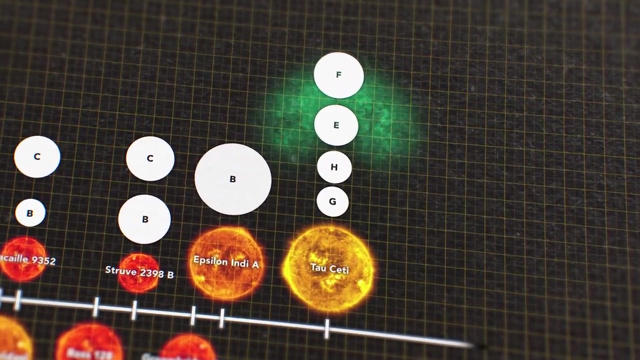 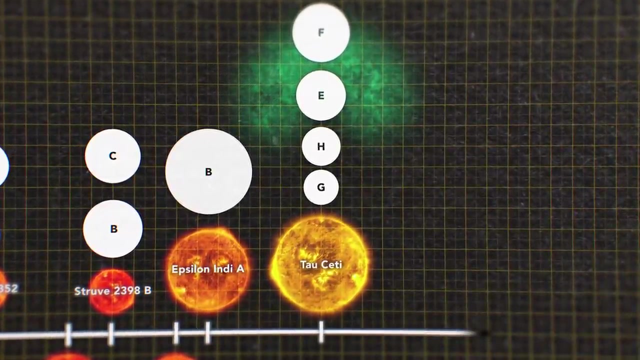 good sign, but far from a sure thing. While, as of now, a lot remains uncertain about this system, the sheer number of planets expected to be found here, paired with the star's similarity to ours, has driven continued interest around these alien worlds. The two other more Earth-sized planets, Tau Ceti G and 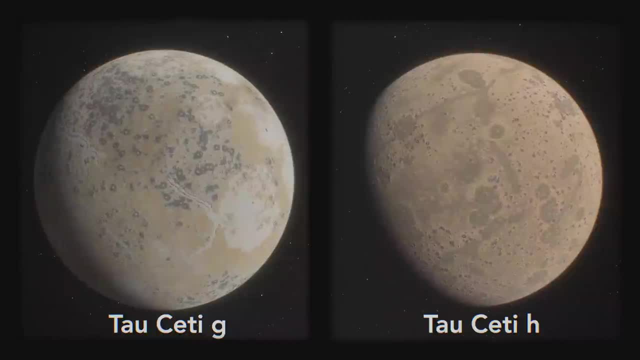 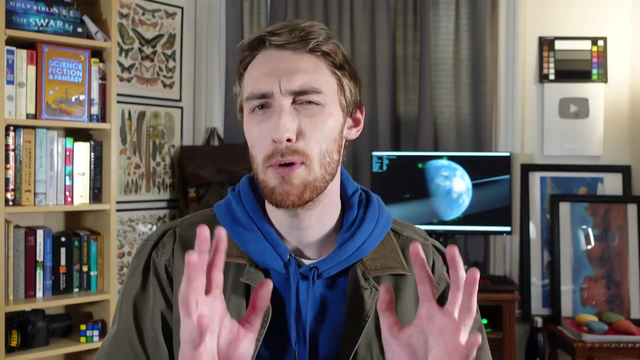 H. both sit far too close to their star and are likely little more than rocky worlds stripped of any atmosphere to the point where I don't really feel bad about skipping over them. But okay, it was at this point in writing my script that 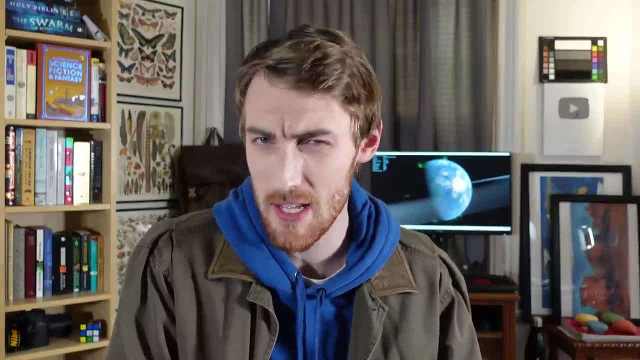 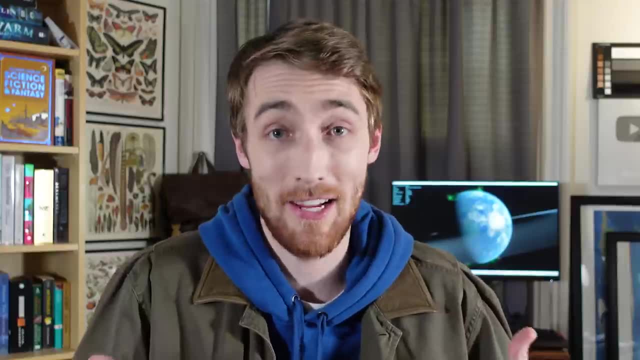 I realized I didn't actually know how to end a video like this. I mean, there are nearly 5,000 planets for us to explore, but there are only so many ways of saying I don't know. we need more information. And plus, I'm kind of aiming to keep this video under. 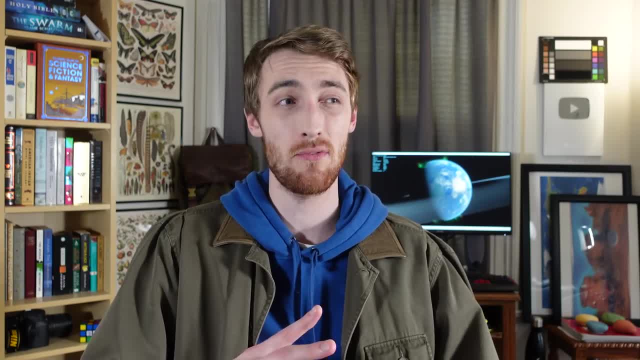 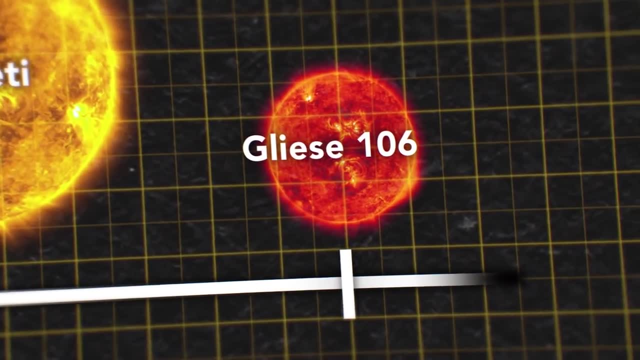 30 minutes, so let's look at one more example and then see if there are any bigger trends we can parse out. The next star with confirmed exoplanets is Gliese 1061, and yes, it's another red dwarf Here. three planets have been. 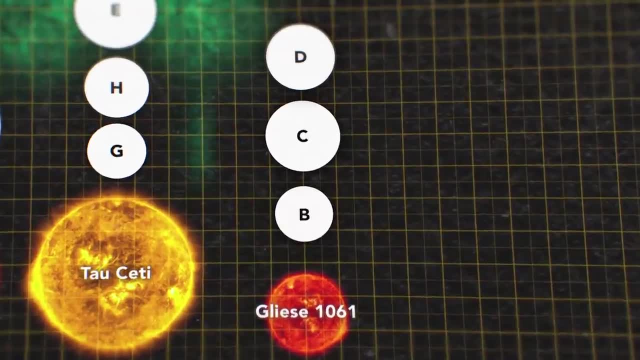 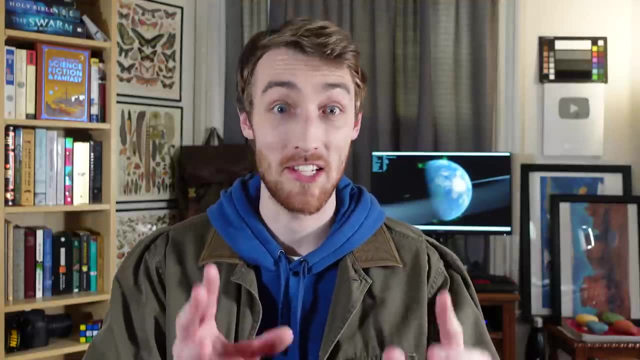 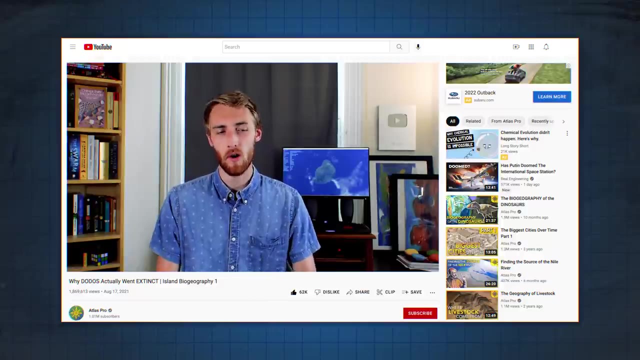 confirmed, all of which are rocky and two of which- Gliese 1061c and Gliese 1061d- orbit within their habitable zone. And this is where things get real interesting, as it opens up the possibility of exchange. You see, lately I've been talking a lot about a field of 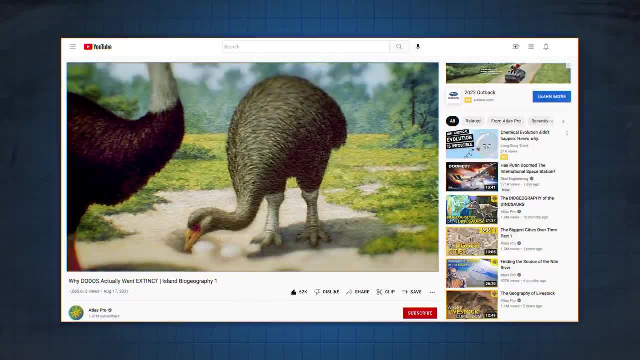 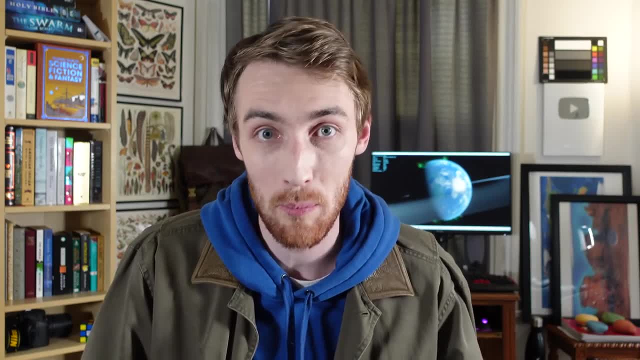 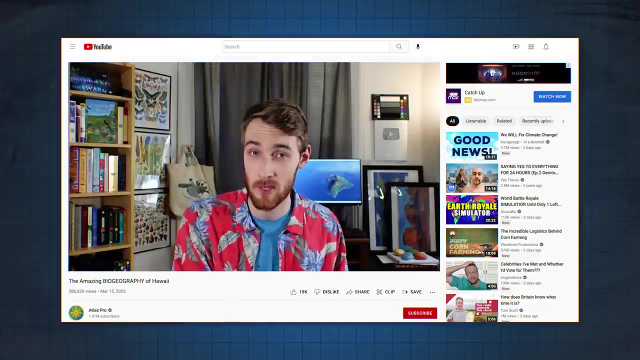 study called island biogeography, and we've been learning how isolation in island environments can have some pretty wild evolutionary effects. And what are planets, if not inherently isolated environments? Yep, that's right, planets are islands. Specifically, in my last video, I described an evolutionary process called adaptive radiation. that 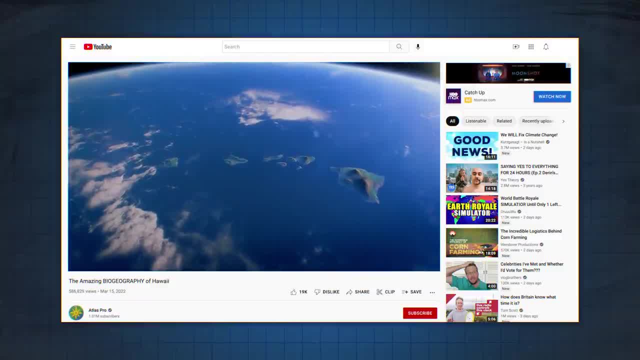 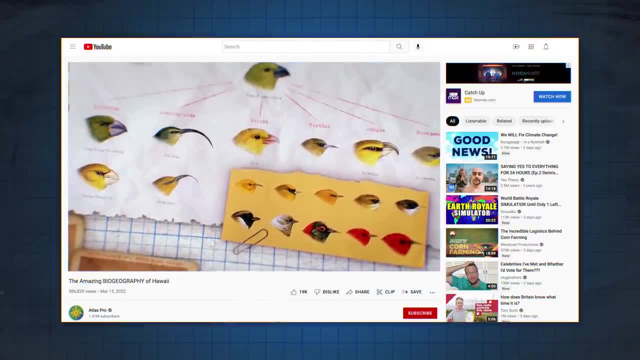 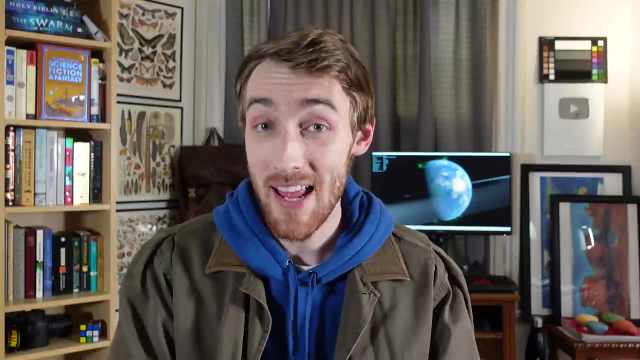 here on Earth occurs when an organism finds a new environment with unfilled niches, like an island. Over time, the advantages of filling these niches leads to speciation, producing a variety of different organisms or species, all with one common ancestor. But now I want to talk a little bit more about the 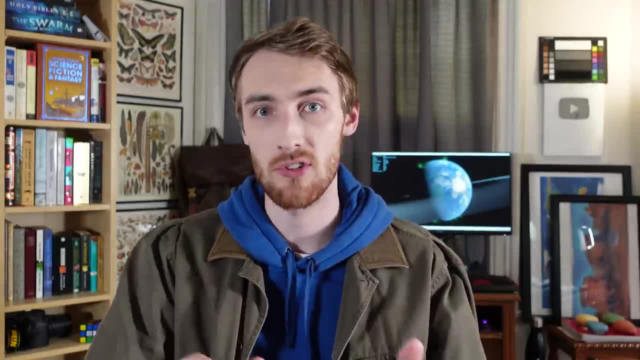 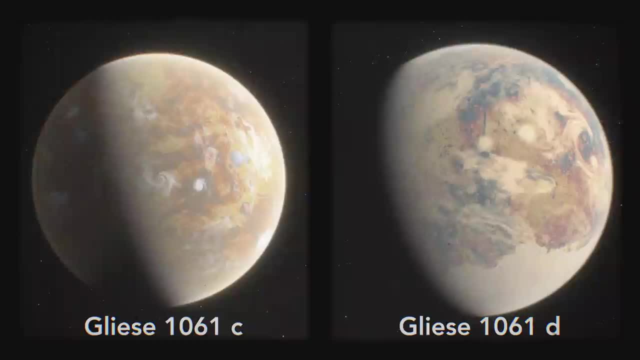 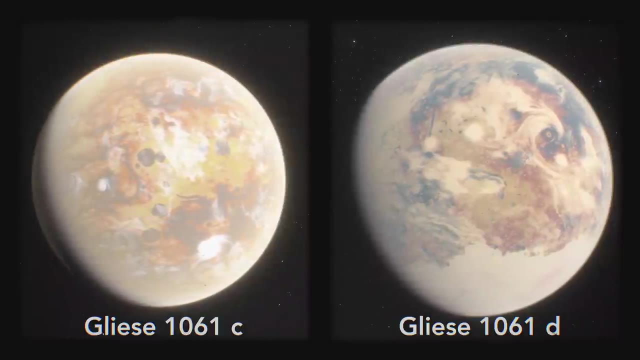 evolution of life. I want to apply this evolutionary model to extraterrestrial life, a field of study I think is only fitting to call astro-bio-geography. In the simplest of scenarios, like what we'll find around Gliese 1061,, we'll have two planets, both capable of supporting some form of life. 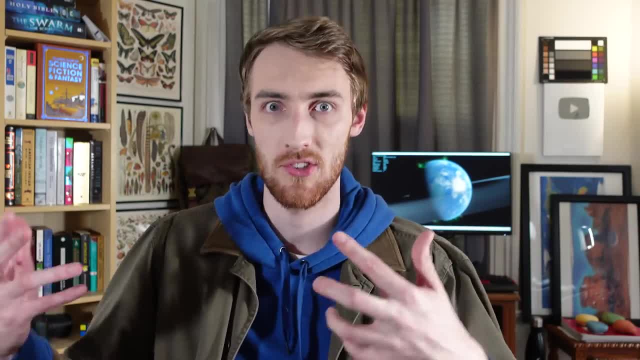 But hang on, to save myself the trouble of saying Gliese 1061c and 1061d over and over and over again. how about we call them something like I don't know, something like Gliese 1061d? 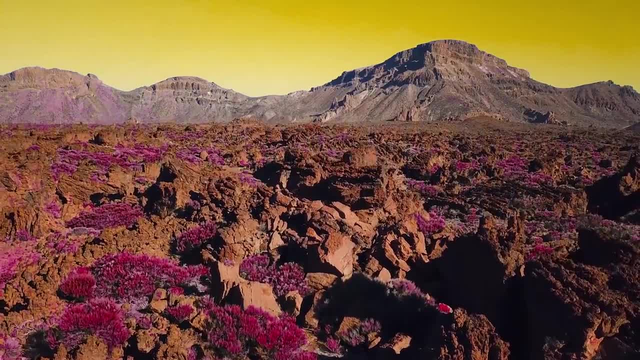 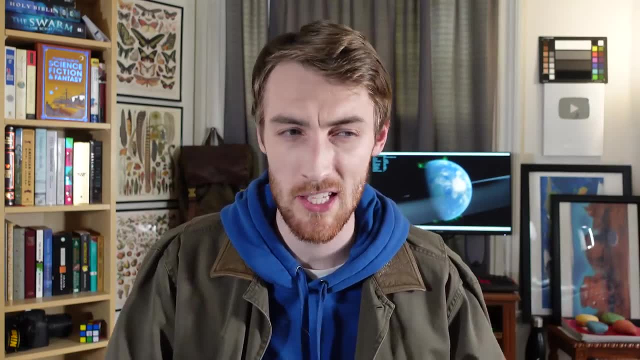 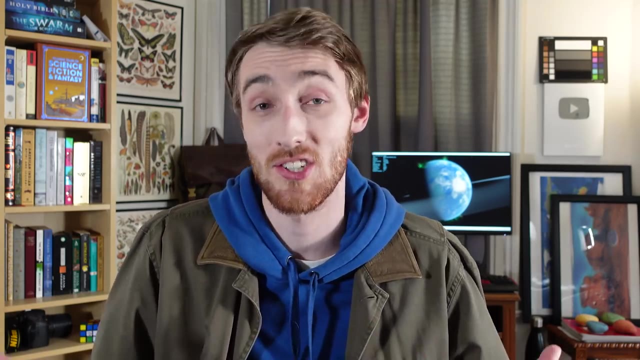 Chippendale. With so many factors at play, it's really anyone's guess as to which planet life would develop on first. But considering everything else even, it's my guess that life would more readily develop in a warmer environment than a colder one, though that's just a hunch. Either way, it's almost a sure thing that. 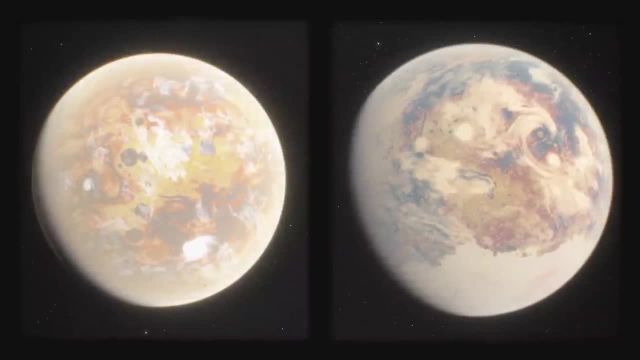 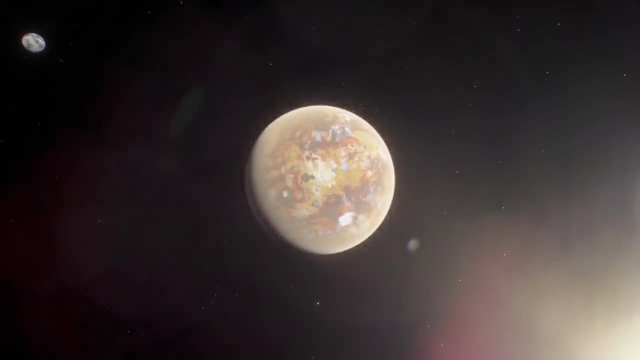 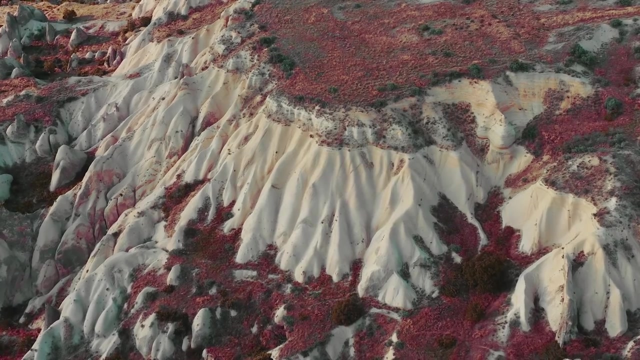 life would start on one planet before the other. For our purposes, let's just say, Chip's position closer to its star allows it to develop the first biology in the system Like this. Chip essentially serves as this system's mainland. From here, the only conceivable way for life from Chip to migrate to Dale would be some. 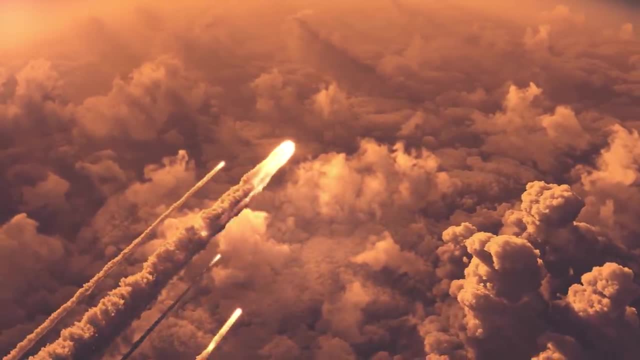 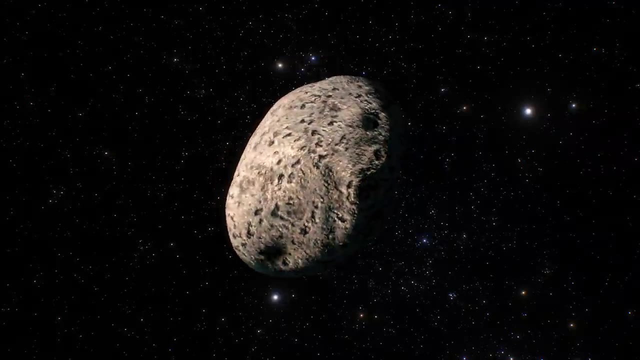 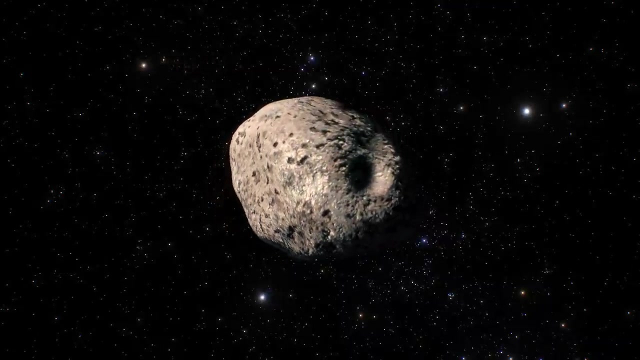 sort of random impact event, an asteroid collision that kicks up a bunch of material from Chip's surface into space. This mechanism for planetary colonization limits migration to only the most simple, most resilient of microbes, as these would have the best and really only chances of surviving their potentially decades. 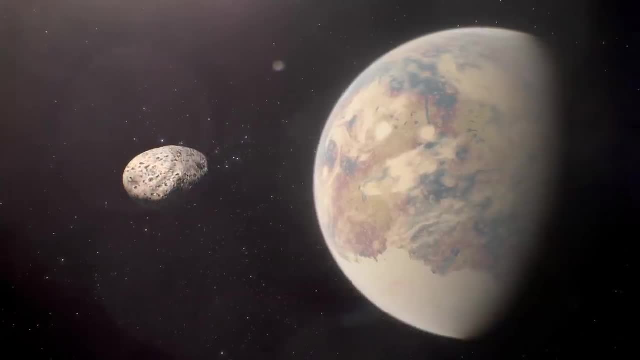 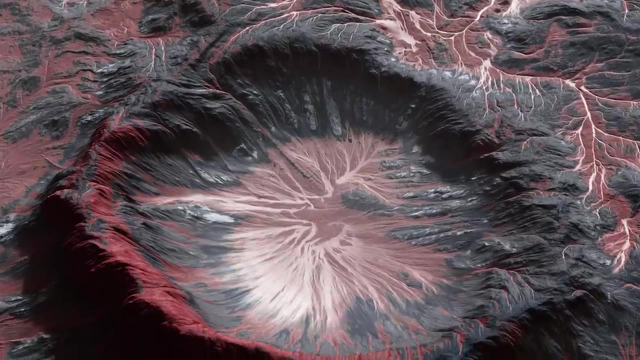 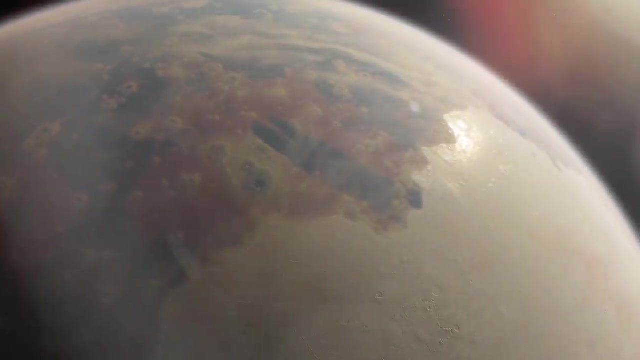 long voyage on an asteroid. Nevertheless, if some of this material finds its way to Dale and survives re-entry into the atmosphere, it will have successfully seeded the planet with Chippian life. Except here on Dale, the environment isn't quite the same. It's colder, the gravity's weaker, there's probably a 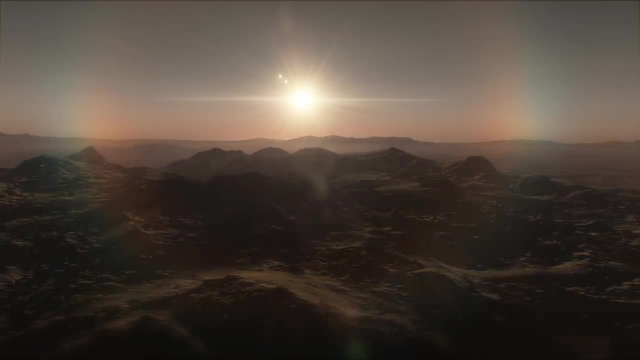 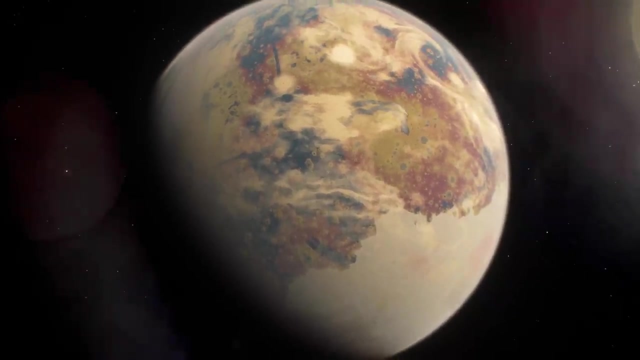 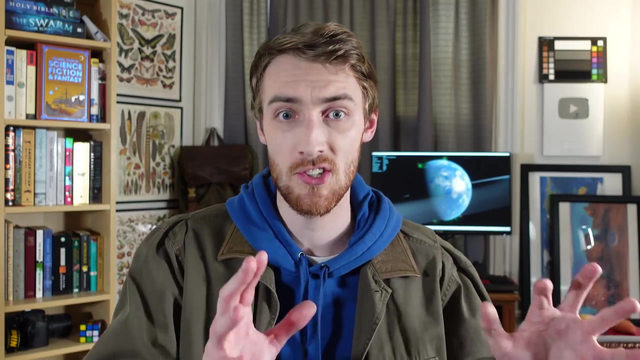 different balance of gases in the air, a different makeup of soils, etc. But if a microbe can survive the harsh environment of space, then it'll probably do just fine under different conditions, so long as nothing here's too toxic. Since we all still have our optimist hats on, let's just say there are no other significant 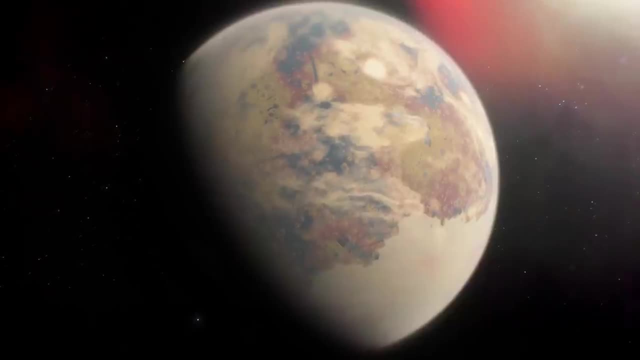 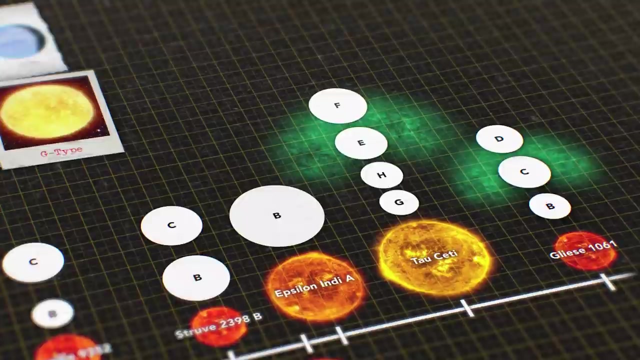 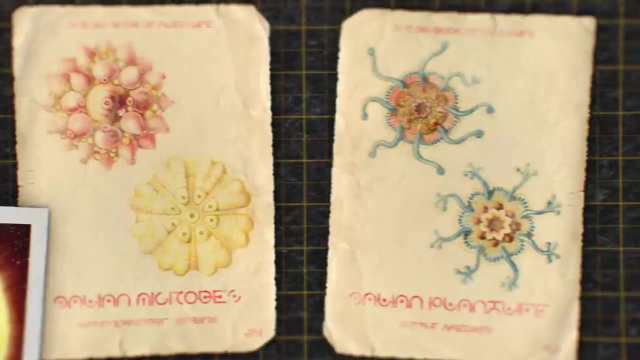 barriers to colonization. besides dispersal From here, Dalean life will spread to all viable corners of the planet and begin its own evolutionary journey, Starting from just a microbe over millions to billions of years, all the various forms of complex life like plants, animals, fungi and everything in 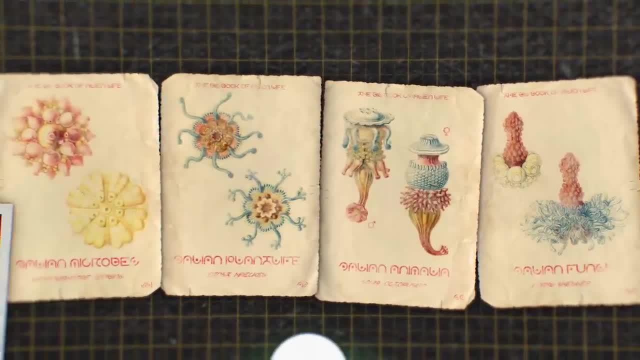 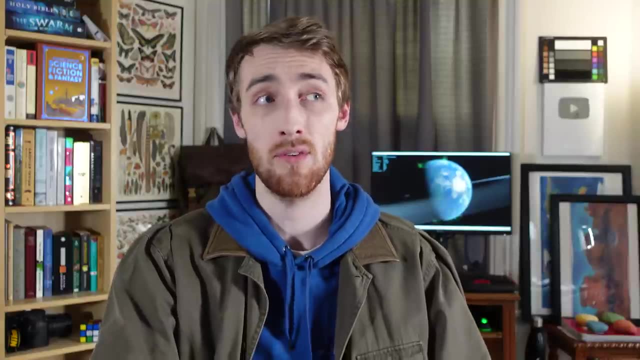 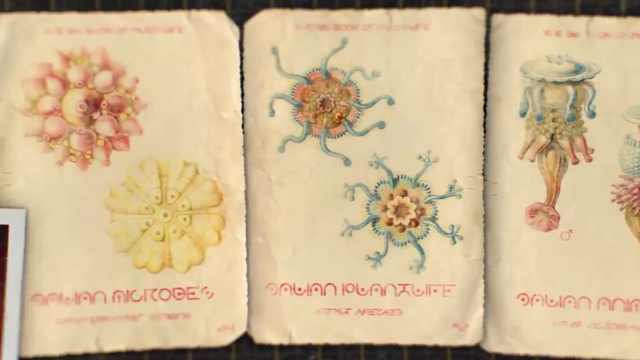 between would arise, the same way it did here on Earth. In this way, planetary colonization represents possibly the most extreme example of adaptive radiation there is, where an entire ecology develops from a single source organism, And this is actually a good place for us to stop. The next star, YZ. 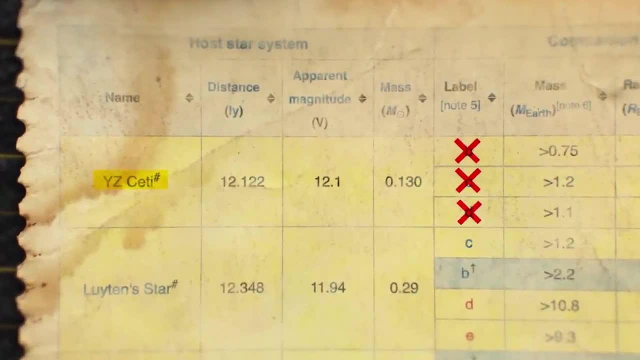 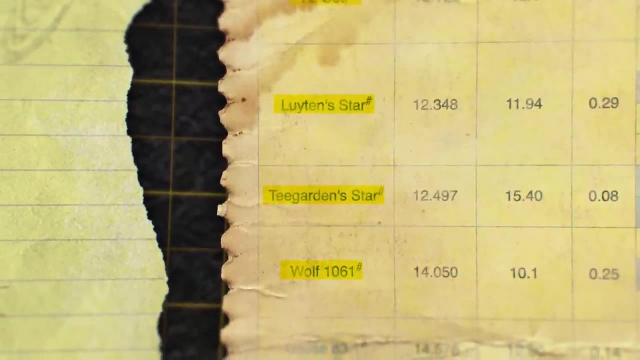 three rocky worlds, which all orbit too close to be considered habitable, and then after that, we'll run into Leighton's star, Teegarden's star and Wolf 1061, all three of which I already covered in my first exoplanets video. So now let's take 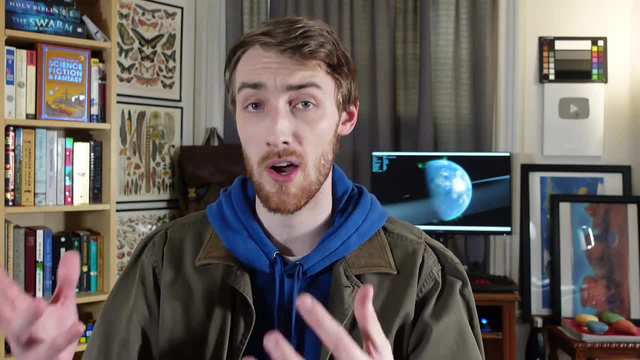 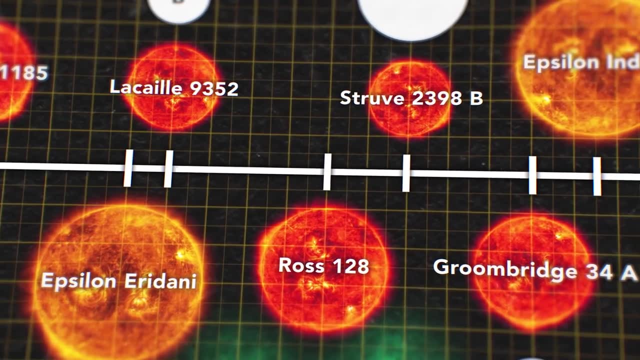 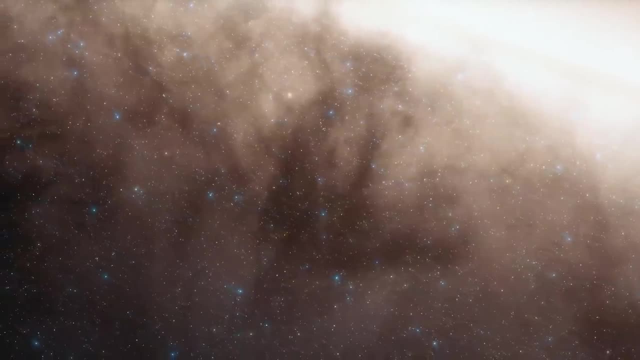 what we've observed and try to come to some conclusions on our cosmic neighborhood. I think the first thing we must all be aware of by now is the clear prevalence of red dwarf stars. As it turns out, the smaller in mass a star type is, the more common. it is explaining why over 75% of all the stars in the 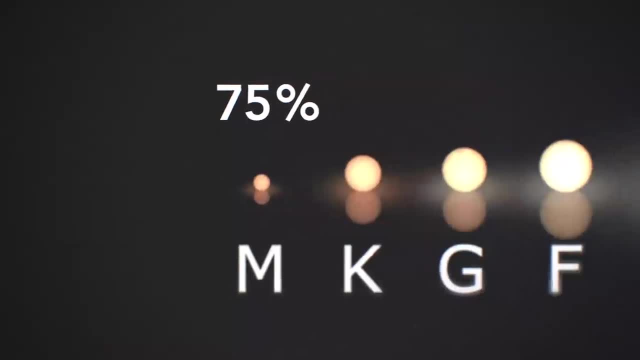 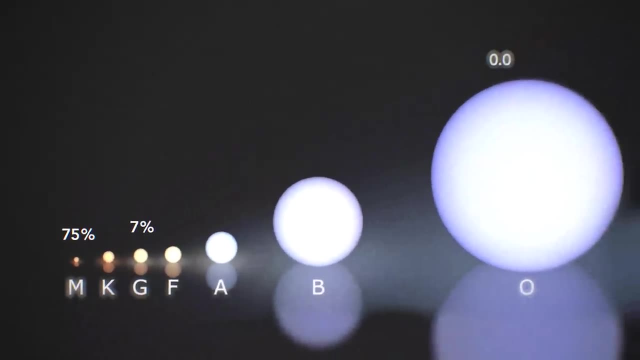 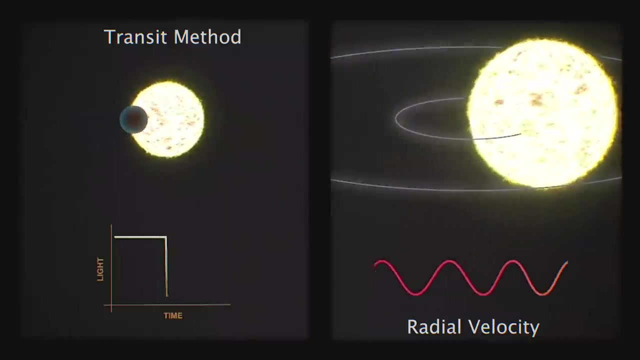 universe are red dwarfs, with bigger g-type stars like ours coming in at only 7%, and the biggest O-types being exceedingly rare, at 0.00003%. On top of that, their smaller size and dimmer stars are the ones that are the most common stars in the universe. 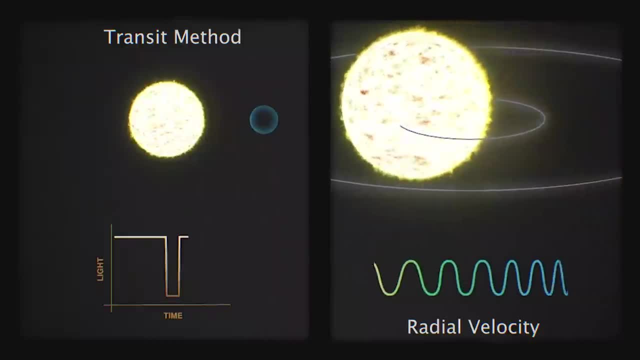 On top of that, their smaller size and dimmer stars are the ones that are the most common stars in the universe. On top of that, their smaller size and dimmer light makes detecting planets around them far easier than any other star type, meaning there's also likely a 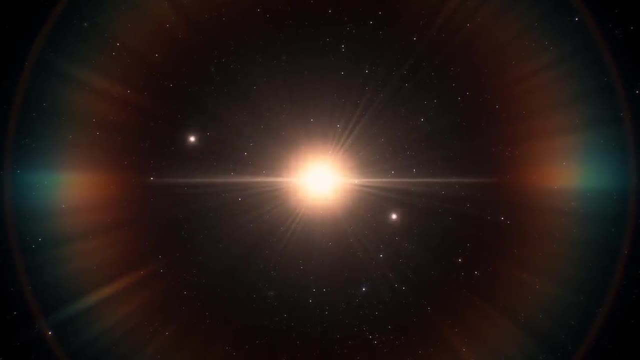 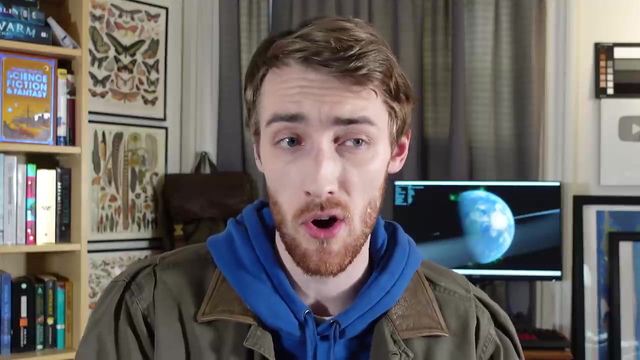 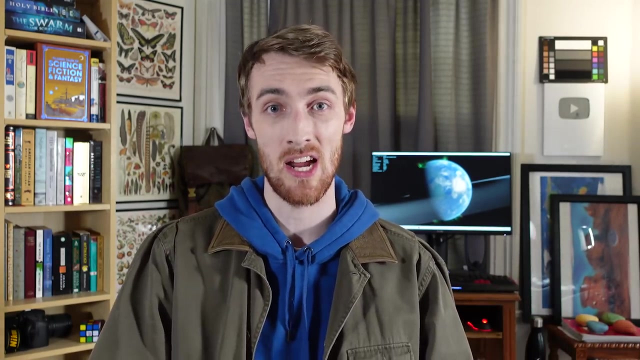 large bias in our data set towards red systems. The second thing I noticed and found surprising was just how many of the planets we've discovered are rocky or terrestrial. Going into this video, I was fully expecting most of them to be gas giants, simply because they're bigger and therefore easier to find, but it would. 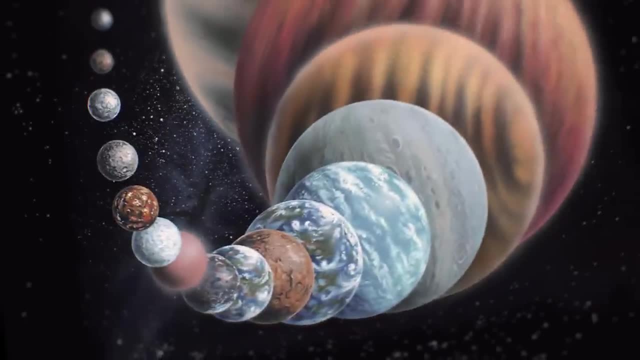 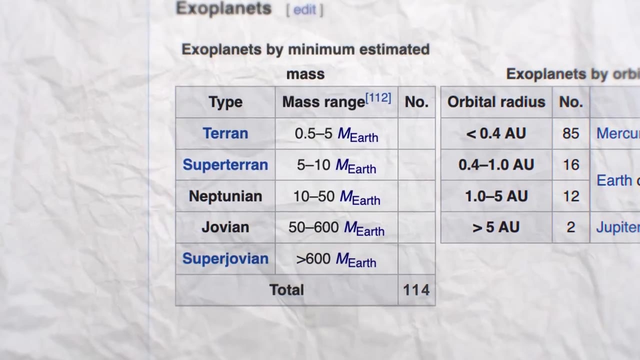 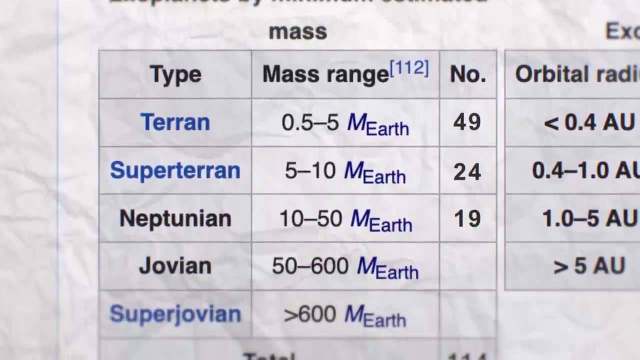 appear that most star types are not. Most star systems feature a balance of rocky and gaseous planets. In fact, if we tally up all 114 exoplanets listed on the Wikipedia page, 49 of them appear terrestrial, 24 were super terrestrial, 29 were Neptunian, 10 were Jovian and only 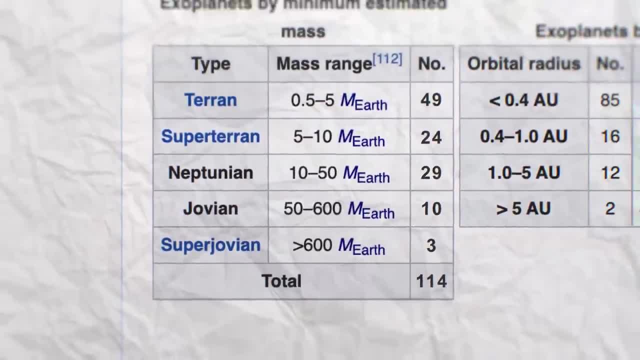 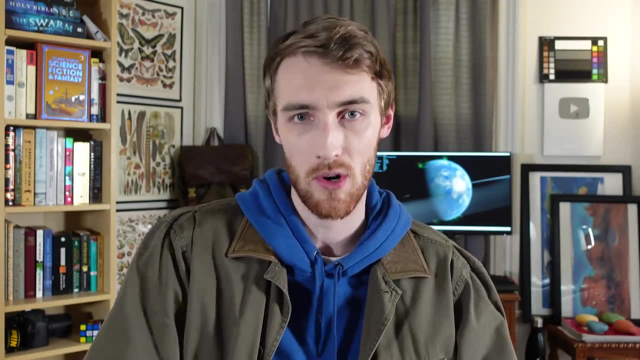 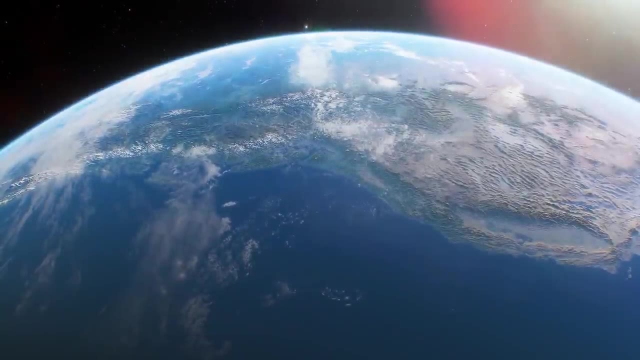 three were super Jovian, showing a clear tendency towards smaller planets. Thinking about it now, this just makes sense. the same way, how smaller stars are more common stars? Luckily for us, smaller rocky planets also just so happen to be the only known places. 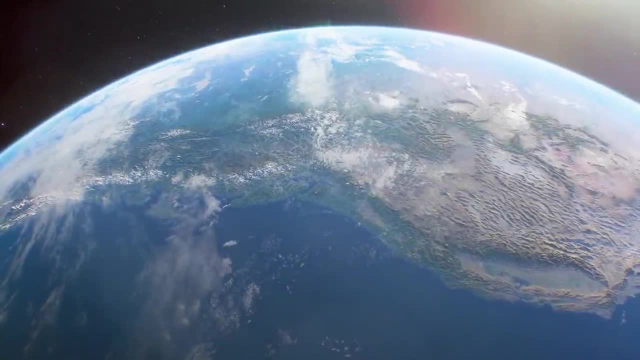 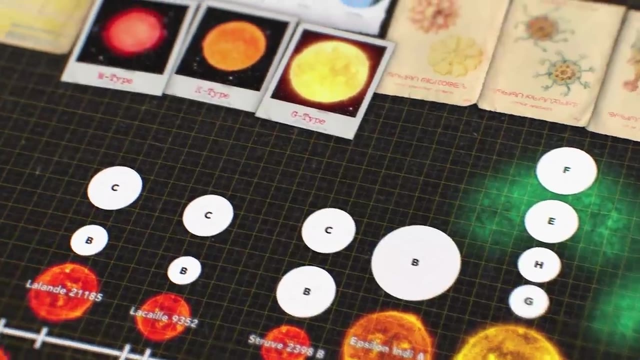 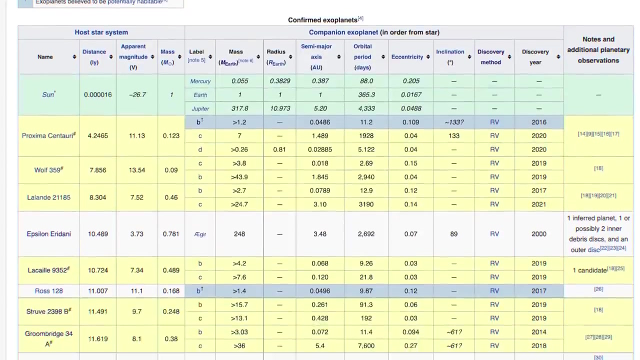 to support life, making our chances of finding more Earth-like planets pretty good. Lastly, I wanted to look into the math a little. In total, we ended up looking at 12 star systems, four of which hosted at least one potentially habitable planet. Expanding this to the nearest, 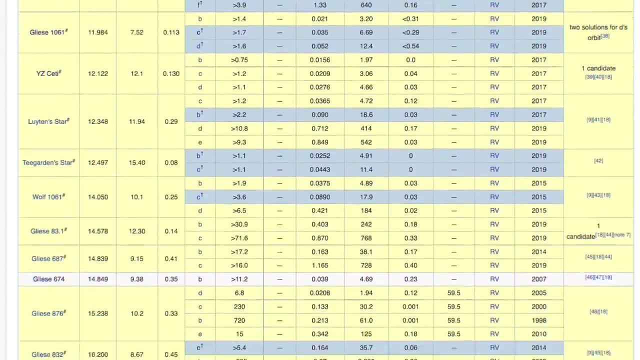 57 star systems. we found that the total number of planets in the world that are more likely to have a habitable planet is 14 star systems, or all the ones listed on the Wikipedia page. a total of 14 hosted rocky planets within their habitable zones, or roughly a quarter. 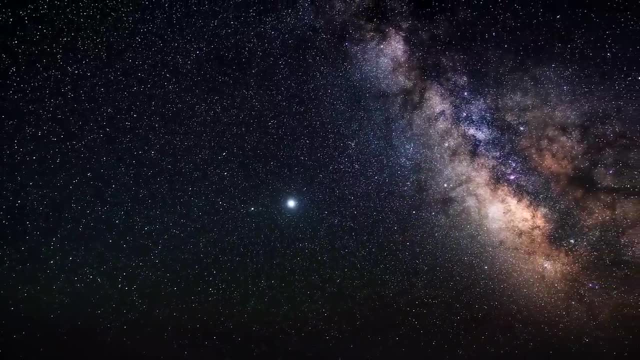 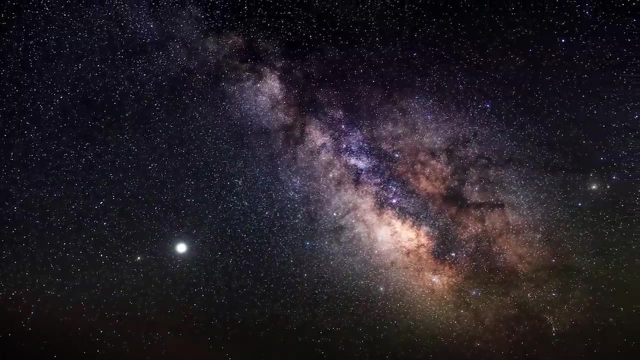 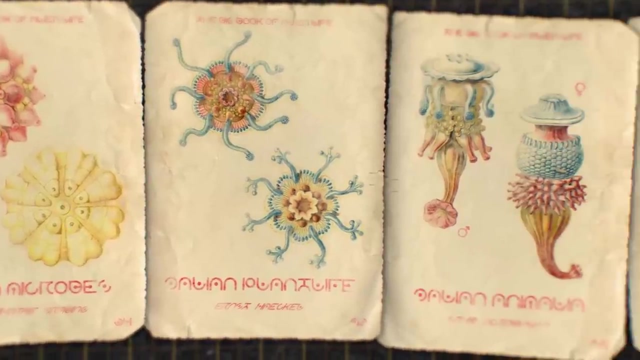 of them, While, of course, this list is constantly being updated. if these numbers hold and anywhere near 25% of all star systems host even potentially viable worlds, not only is this a remarkably high number, but also means we might not need to look all that far away to find some form. 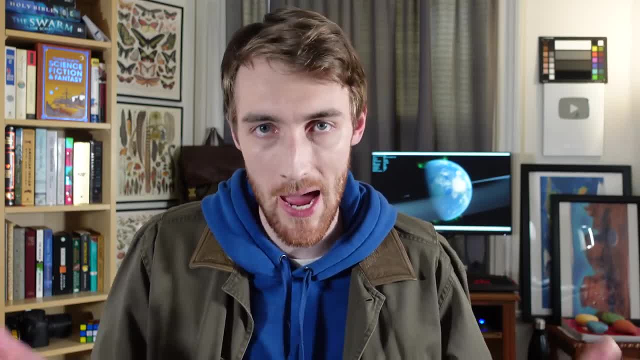 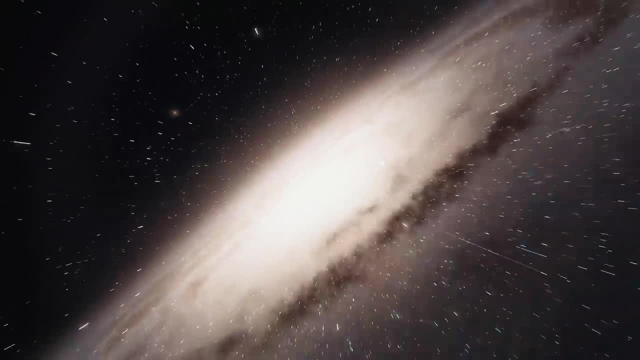 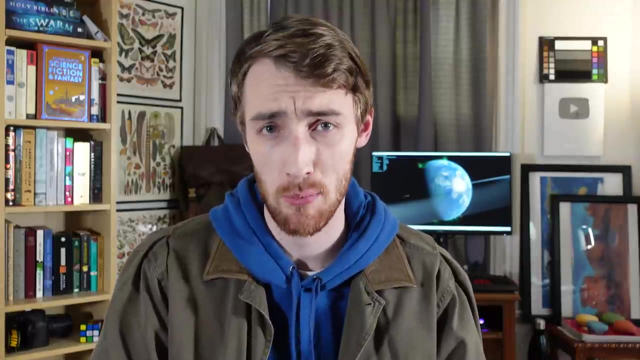 of alien life. Now, sure, not all of these will be habitable, but even if just a fraction or a fraction of a fraction of them are, that would still amount to millions of living worlds in the Milky Way alone. And I think that's what I find to be the most exciting part of studying exoplanets: If we